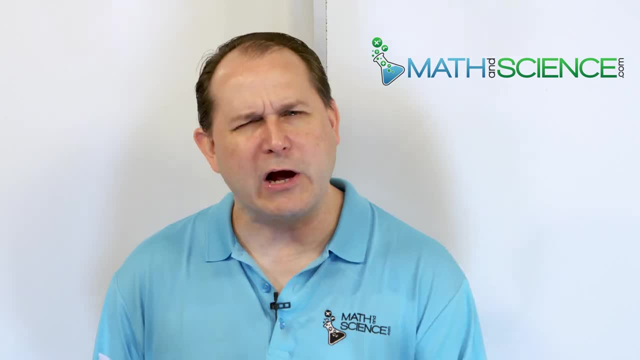 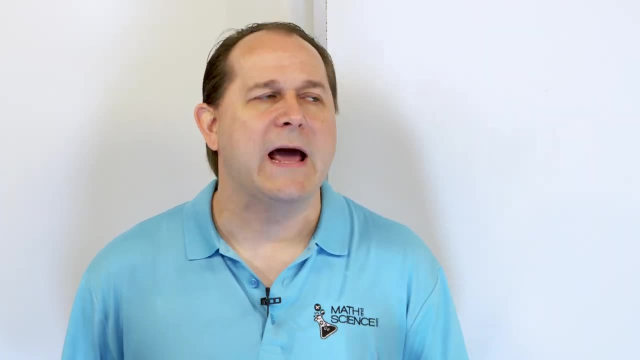 attention to understanding some definitions. They look very complex, but they're actually very simple to understand and you need to know them because, as we move on into further material I will talk about: hey, what is the third term of that expression? What is the fourth variable? 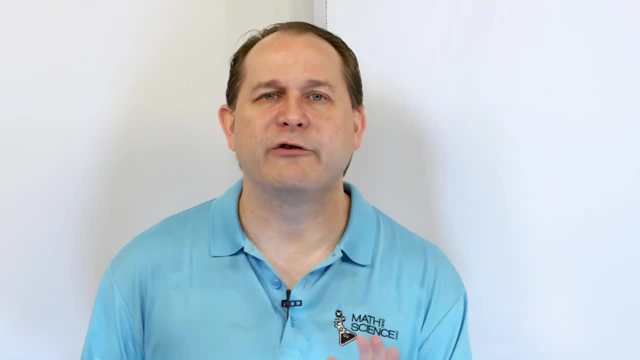 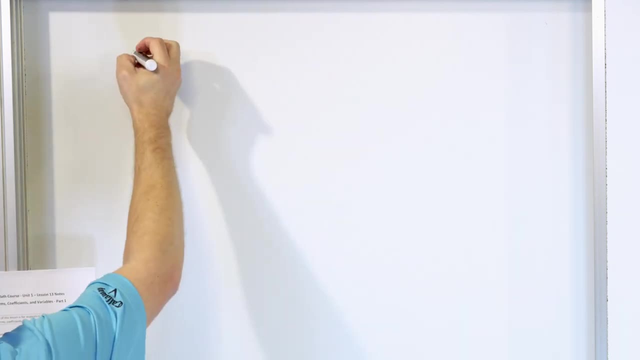 over there And you need to know in your mind what is it really talking about. So here is where we learn what I'm talking about, right, All right. so let's learn by example. I'm not going to give you a bunch of definitions, I'm just going to show you what this basically means. Let's say I have 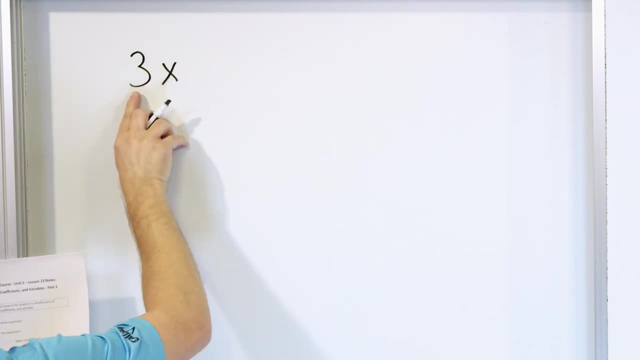 something like this: 3x. Now notice this: when I put a number right next to a letter and there's nothing in between them, that means they're multiplied together. I could put a dot right there for 3 times x, but you can't do that, So I'm going to put a dot right there for 3 times x. 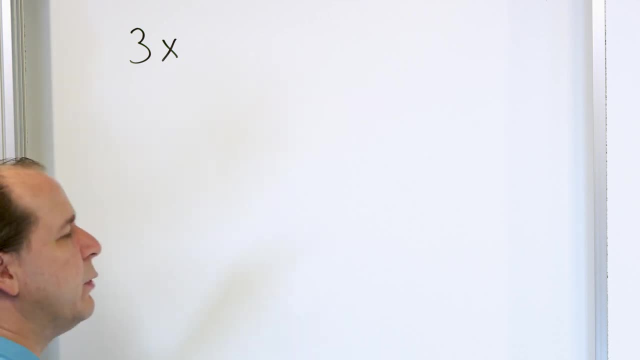 but you need to learn that when you see a number right next to a variable, it means they're multiplied together. So 3x means 3 times x. You're no longer going to be writing the multiplication symbol between numbers and variables, So this means 3 times x. Whatever x is, I'm just going. 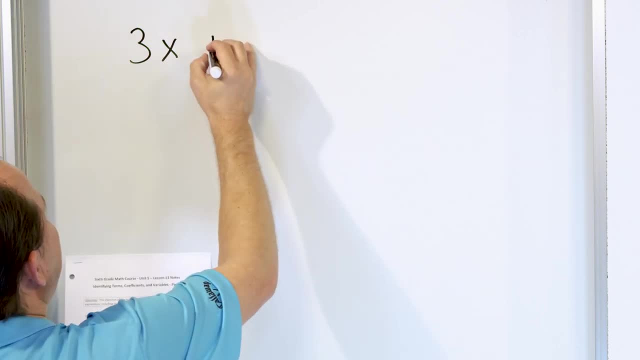 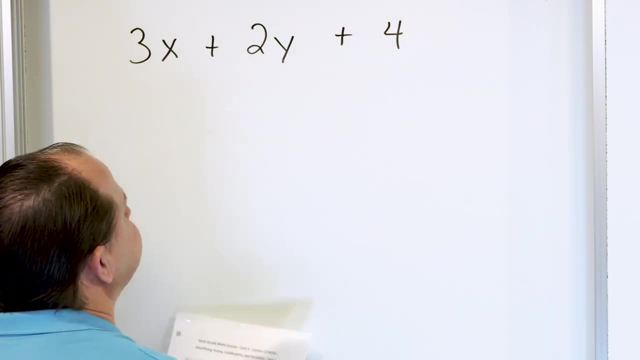 to triple it. That's all it means, okay. And then I'm going to add to that 2 times a totally different variable, y, And then I'm going to add to that the number 4, all right, So this whole. 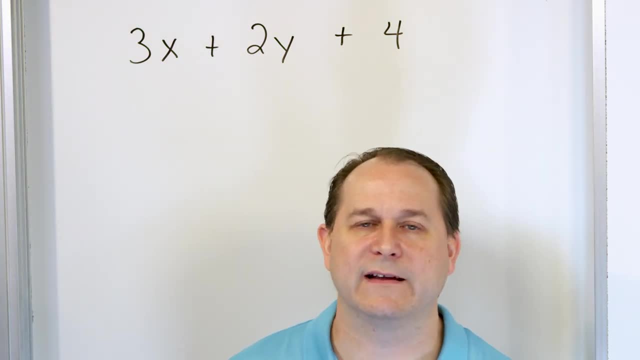 thing is what we call an equation, So I'm going to add to that the number 4,. all right, So this whole thing is what we call an expression. We learned about that in the last lesson. It's an expression because it's not an equation. An equation has an equal sign somewhere There's no. 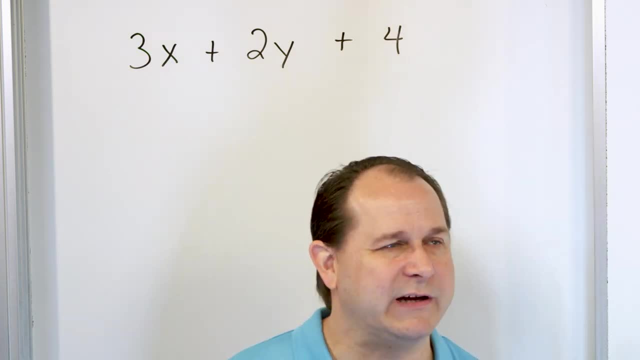 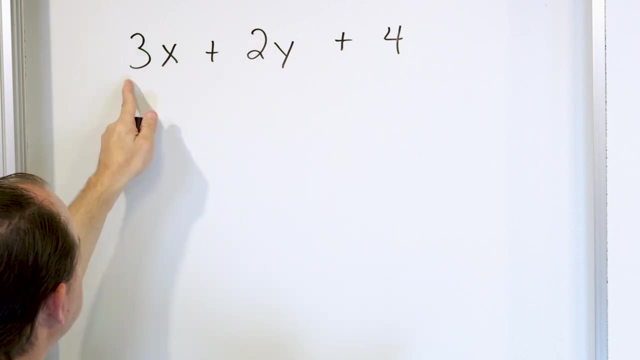 equal sign here. So this is an expression. It means it's a calculation. If I tell you what x is and you stick it in here, and I tell you what y is and you stick it in here, then I can multiply and then multiply and I can just add it all up and calculate the answer. So that's an expression. 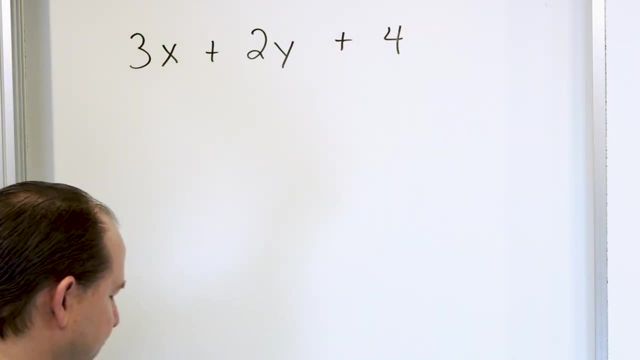 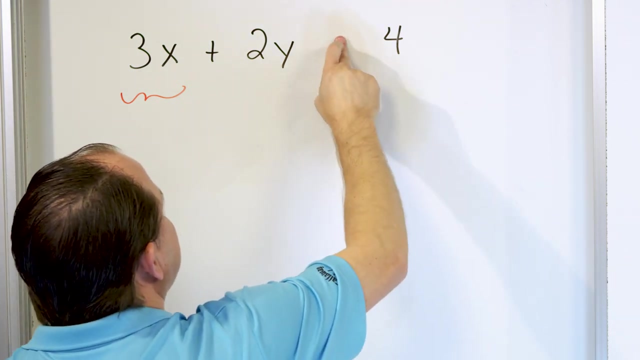 Expression is a calculation. Now we're going to dive a little deeper into learning some definitions. All right, so what we have here is this kind of thing, all the things linked by the plus signs, I guess to make it kind of different, it doesn't have to have plus signs everywhere. I 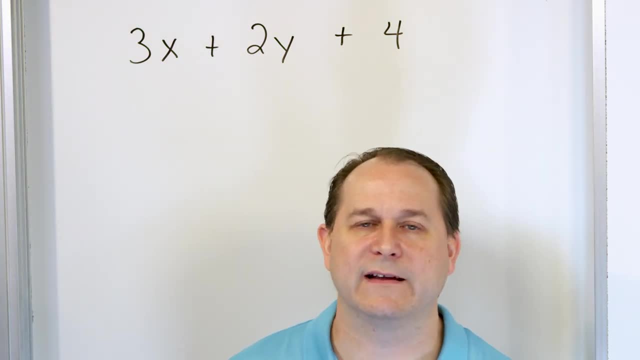 thing is what we call an equation, So I'm going to add to that the number 4,. all right, So this whole thing is what we call an expression. We learned about that in the last lesson. It's an expression because it's not an equation. An equation has an equal sign somewhere There's no. 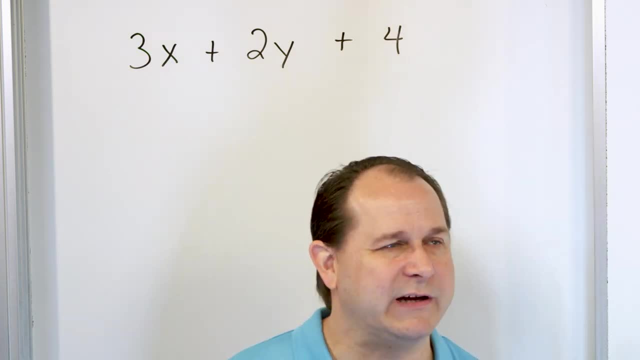 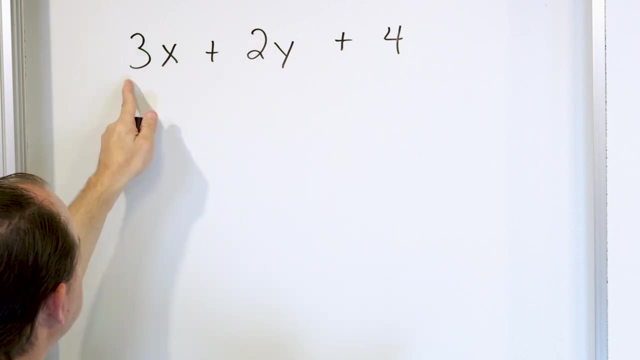 equal sign here. So this is an expression. It means it's a calculation. If I tell you what x is and you stick it in here, and I tell you what y is and you stick it in here, then I can multiply and then multiply and I can just add it all up and calculate the answer. So that's an expression. 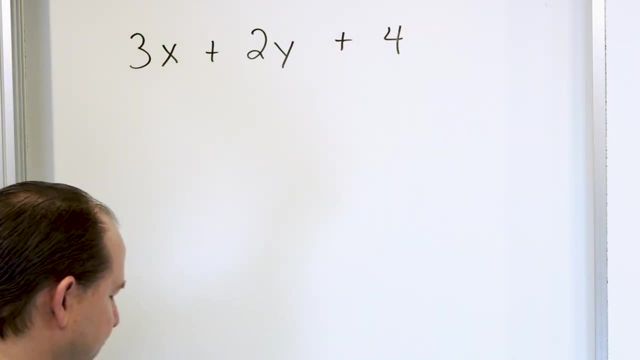 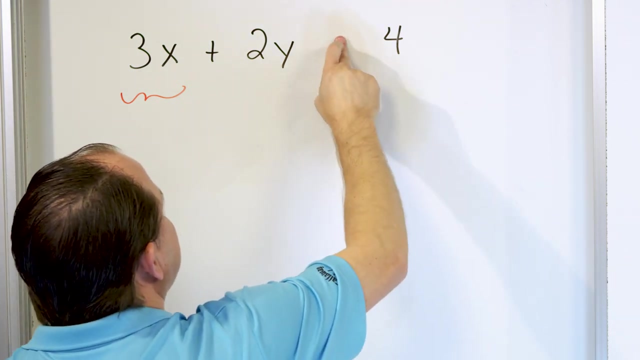 Expression is a calculation. Now we're going to dive a little deeper into learning some definitions. All right, so what we have here is this kind of thing, all the things linked by the plus signs, I guess to make it kind of different, it doesn't have to have plus signs everywhere. I 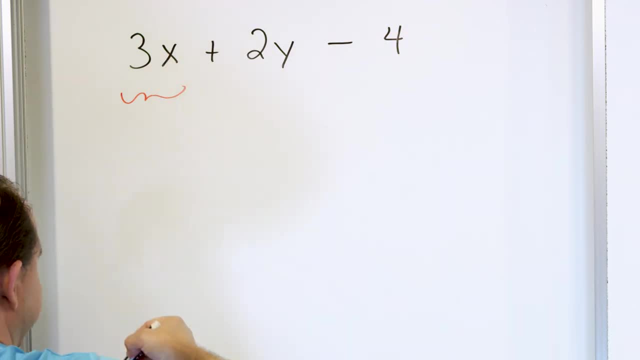 can just change this one, that minus sign. It doesn't have to be plus signs, plus or minus signs, The things that are linked together by plus or minus signs, these are called terms. So this is a term, right, This is also a term, And this one down here is also a term, And this one. 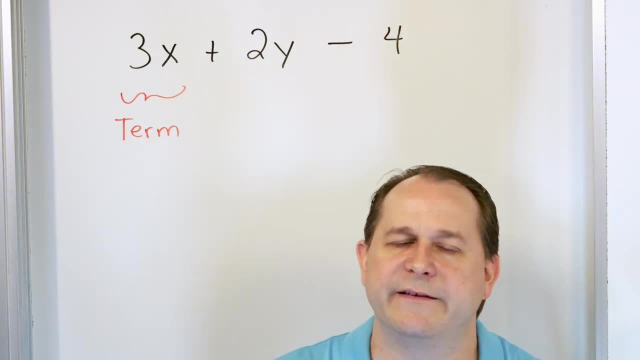 down here is also a term. So the things that are linked together by plus or minus signs, the groupings of things, whatever they are in front of the plus or the minus signs, those are called terms. So if I say what's the first term in this expression, you'll say three x. That's the first. 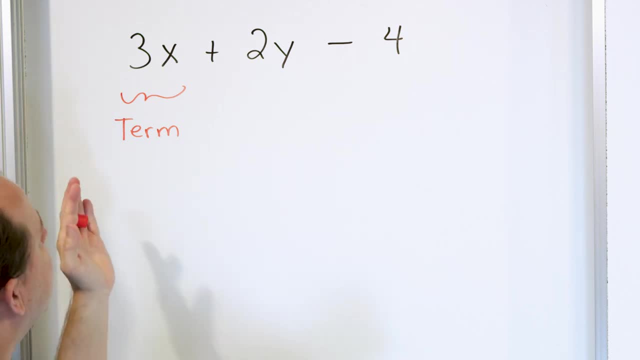 term. If I say what's the third term of this expression, You will go down here and point over here. It'll be really there's a negative sign here. So it'd really be like a negative four. right, If I say what is the second term of this expression, You'll point to the two y, So it's. 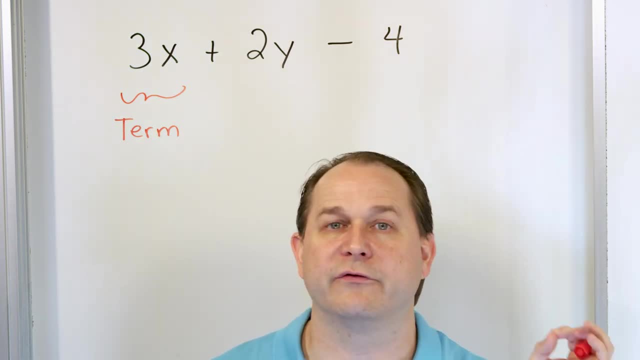 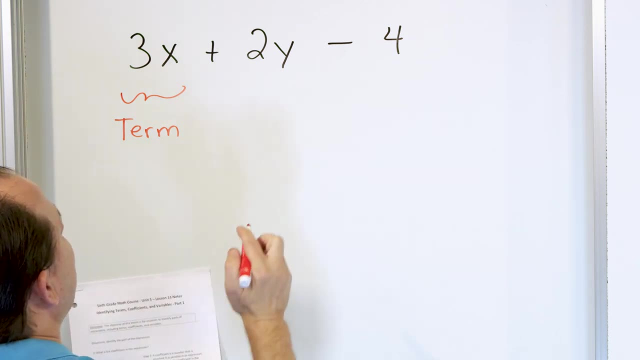 the groupings, It's whatever's in front of the plus or minus signs. Those are called terms. all right, We're going to do a lot of problems, so don't stress out. if you don't totally get it here, Then we of course have the letters. So this is called a variable. 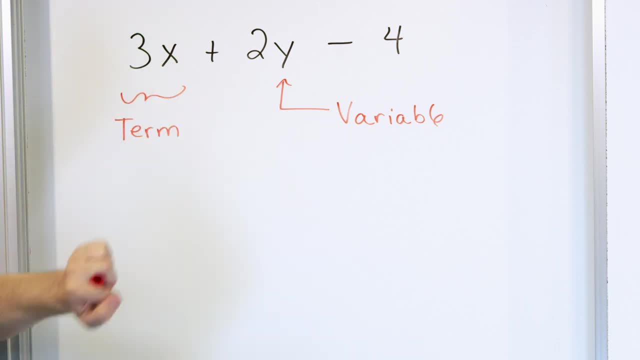 right, We have one variable here, We call it y. We have another variable over here, We call it x. They're totally different things. X could mean the number of pizzas I bake in a week, And y could be the number of muffins I bake in a week. You know, x could be the distance to Mars, Y could be the 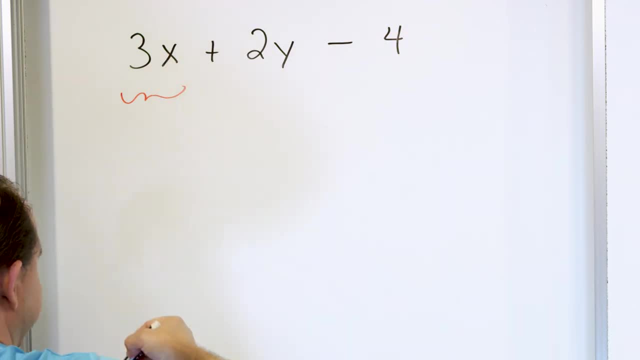 can just change this one, that minus sign. It doesn't have to be plus signs, plus or minus signs, The things that are linked together by plus or minus signs, these are called terms, So this is a term, right, This is also a term, And this one down here is also a term. 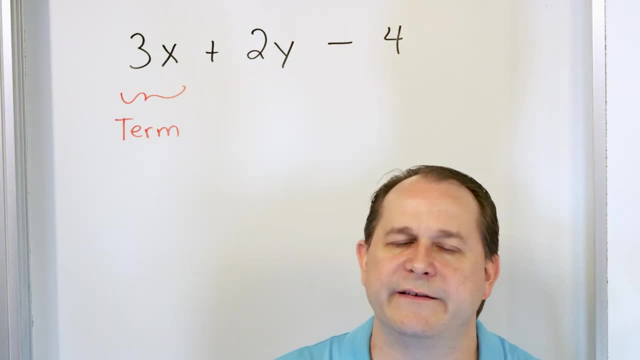 So the things that are linked together by plus or minus signs, the groupings of things, whatever they are in front of the plus or the minus signs, those are called terms. So if I say what's the first term in this expression, You'll say 3x. That's the first term. If I say 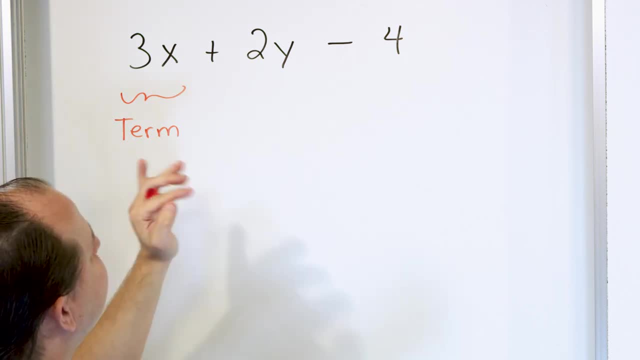 what's the third term of this expression? You will go down here and point over here. It'll be really there's a negative sign here, So it'd really be like a negative four. right, If I say what is the second term of this expression, You'll point to the 2y. So it's the group. 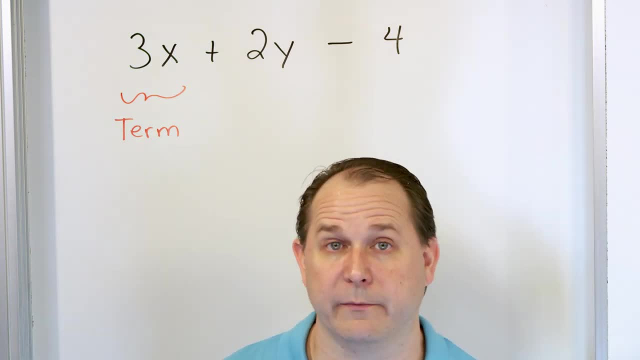 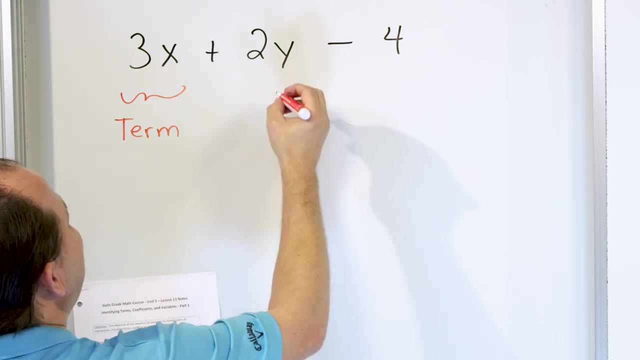 the groupings, It's whatever's in front of the plus or minus signs. Those are called terms. all right, We're going to do a lot of problems, So don't stress out. if you don't totally get it here, Then we of course have the letters. So this is called a variable. 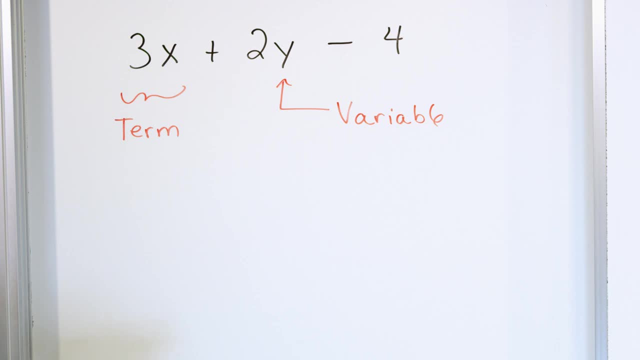 right, We have one variable here, We call it y. We have another variable over here, We call it x. They're totally different things. X could mean the number of pizzas I bake in a week And y could be the number of muffins I bake in a week. You know, x could mean the number of pizzas I bake in a week. 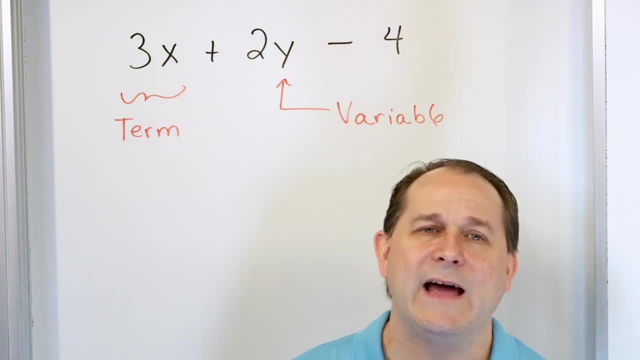 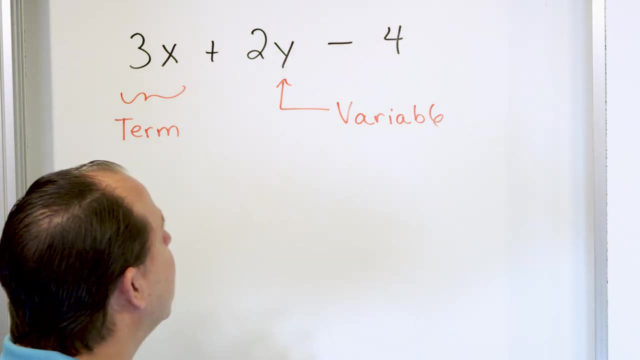 Y could be the distance to Mars, Y could be the distance to the moon. You see the idea. X and y are totally different things. They're different letters and they mean different things. Whatever they mean, they're not the same, They're totally different, right? And then, finally, the last thing. 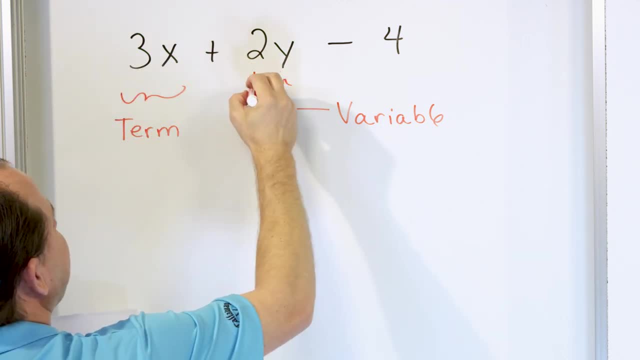 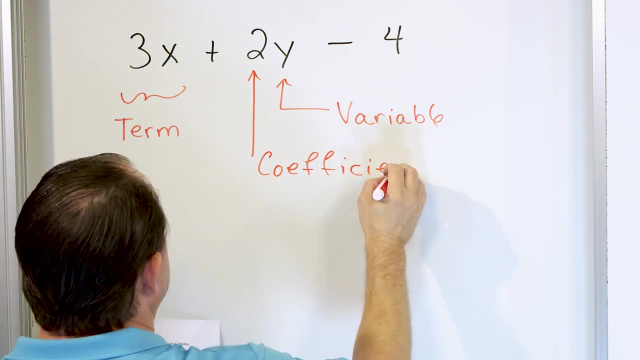 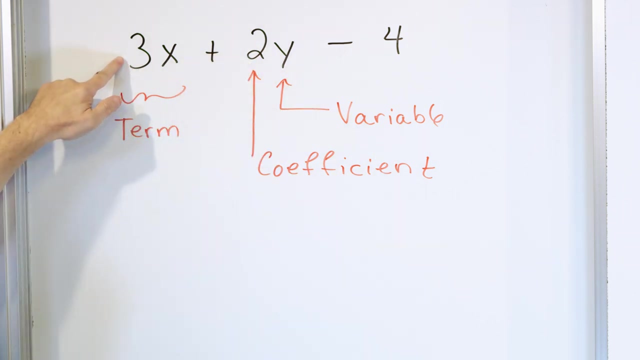 is the numbers that are right in front of their variables. That has a special name also, So this is called a coefficient. okay, A coefficient. So the 2 is the coefficient in front of the y, The 3 is the coefficient in front of the x, And this really isn't a coefficient, because there's no. 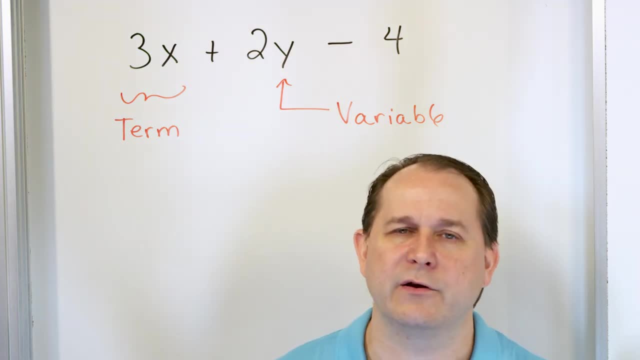 distance to the moon. You see the idea: X and y are totally different things, They're different letters and they mean different things. Whatever they mean, they're not the same, They're totally different, right? And then, finally, the last thing is the numbers that are right in front. 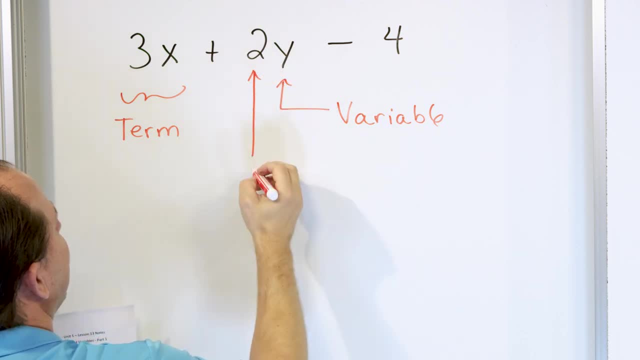 of their variables. that has a special name also. So this is called a coefficient. okay, A coefficient, So the 2 is the coefficient in front of the y, The 3 is the coefficient in front of the x, And this really isn't a coefficient because there's no real variable there. So coefficient. 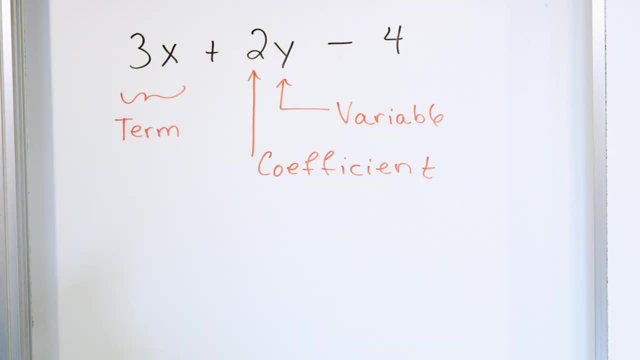 means the numbers that are in front of the letters, essentially. And then to wrap it all up, this entire thing, the whole thing, all the way to the end, we call this an expression, which is what I told you from the beginning. So, basically, the expression is the entire. 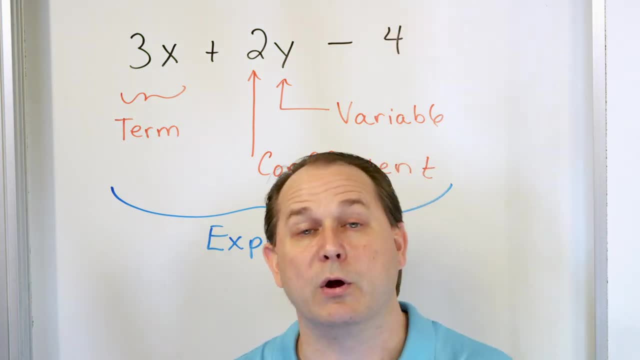 calculation of the number of pizzas I bake in a week. And then the last thing is the number of pizzas I bake in a week. So this is the multiplication you're doing. There's usually pluses, minus signs, multiplication. There can also be division. There can be exponents There. 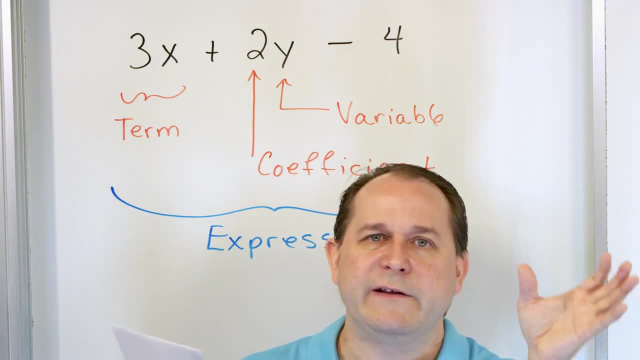 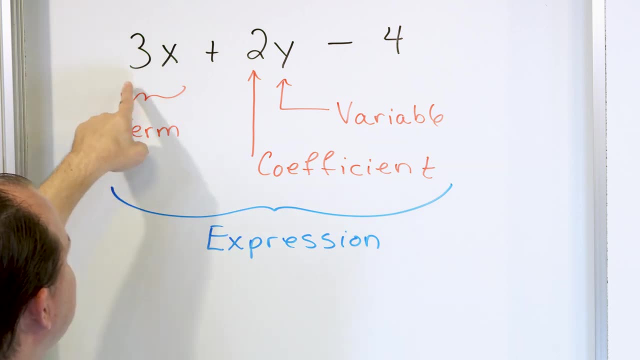 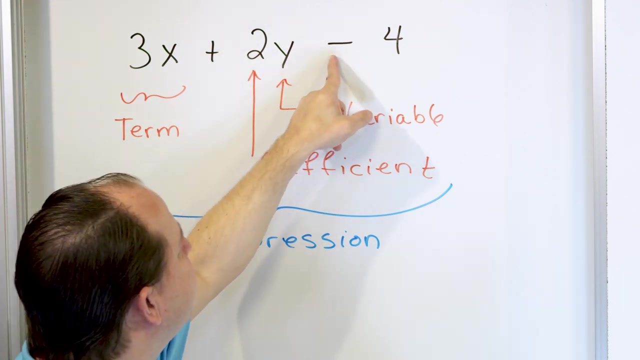 can be other things going on in the expression. Usually there'll be terms that are separated by plus or minus signs, And each grouping of things separated by a plus or minus sign, we call it a term of the expression. This is the first term: 3x. The second term is 2y. The third term is 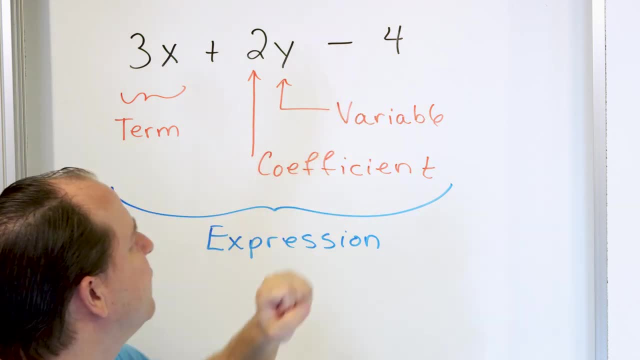 you really include the negative here. the negative 4 would be the third term over here. Then we have what we call variables. Those are all the letters: X is a variable and also y is a variable, And finally the numbers that are right in front of multiplied by the variables. 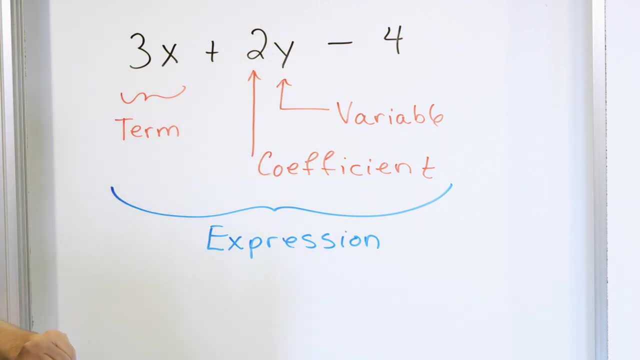 those are called coefficients. So the 2 is the coefficient in front of y and the 3 is the coefficient in front of x. So I know that that's a lot of definitions that we're learning, so we're going to do a lot of problems. right? I'm going to write something on the board. I'm 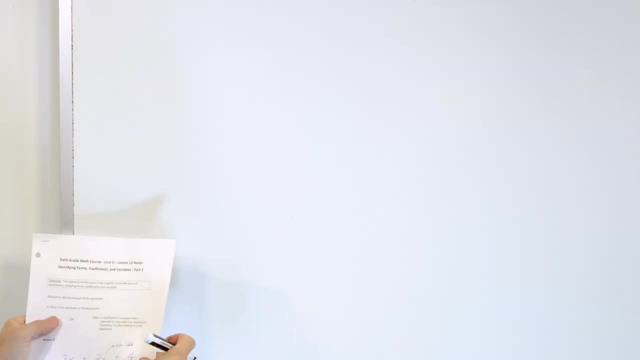 going to ask you a question. So I want you to tell me- here is what I'm writing down: 2x, 2x. I want you to tell me what is the coefficient in that expression. What is the coefficient? So underneath we're going to write coefficient. 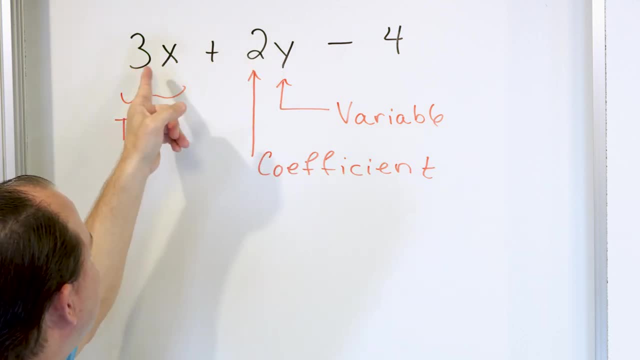 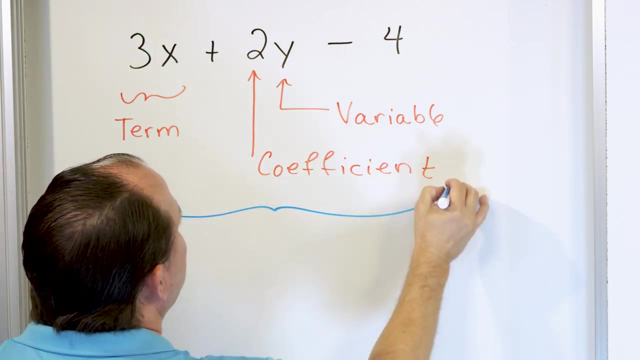 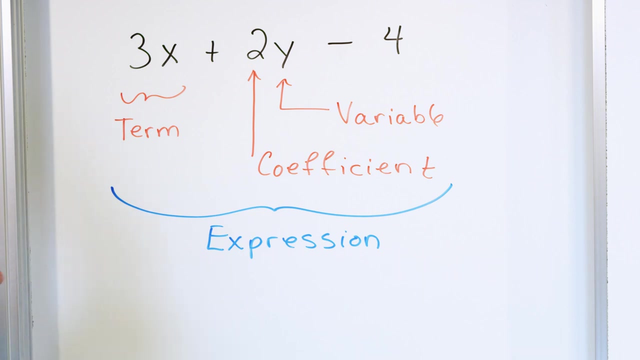 real variable there. So coefficient means the numbers that are in front of the letters, essentially. And then to wrap it all up, this entire thing, the whole thing, all the way to the end, we call this an expression, which is what I told you from the beginning. So, basically, 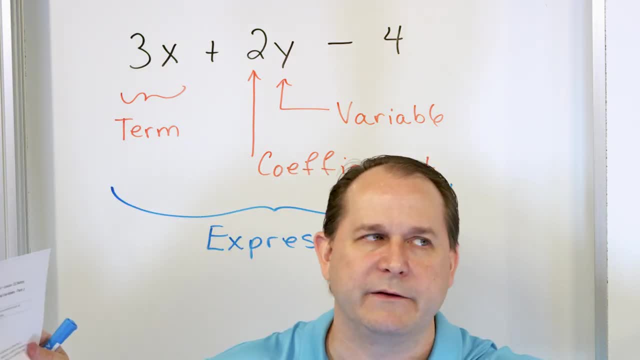 the expression is the entire calculation you're doing. There's usually pluses, minus signs, multiplicators and so on, And then you have the whole thing. And then you have the whole thing. There can also be division, There can be exponents, There can be other things going on in. 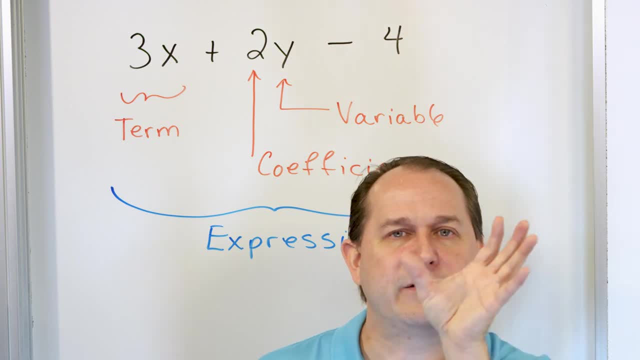 the expression. Usually there'll be terms that are separated by plus or minus signs, And each grouping of things separated by a plus or minus sign, we call it a term of the expression. This is the first term: 3x. The second term is 2y. The third term is: you really include the negative? 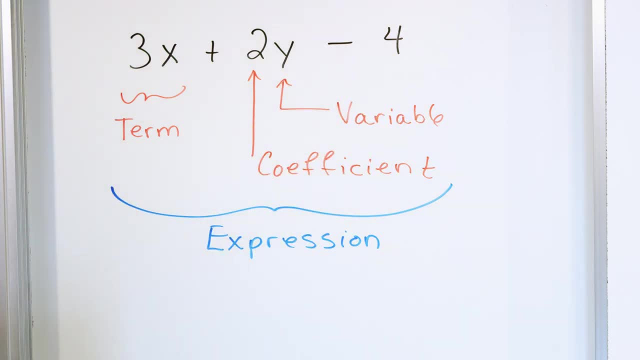 here. The negative 4 would be the third term over here. Then we have what we call variables. Those are all the letters: X is a variable And also y is a variable, And finally the numbers that are right in front of multiplied. 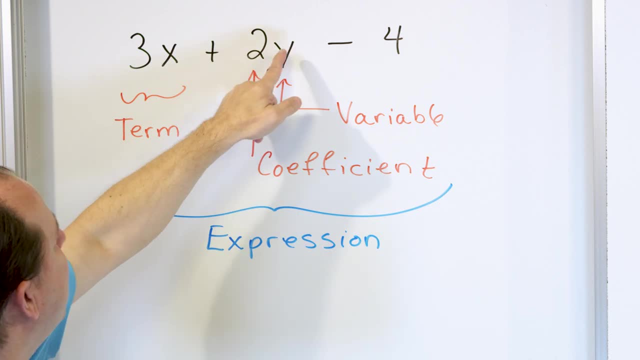 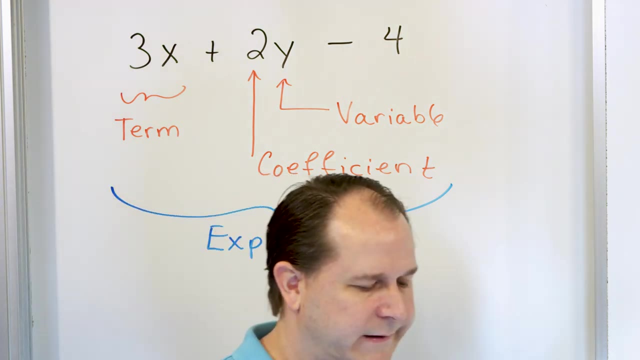 by the variables. those are called coefficients. So the 2 is the coefficient in front of y And the 3 is the coefficient in front of x. So I know that that's a lot of definitions that we're learning. So we're going to do a lot of problems right? I'm going to write something on the board. 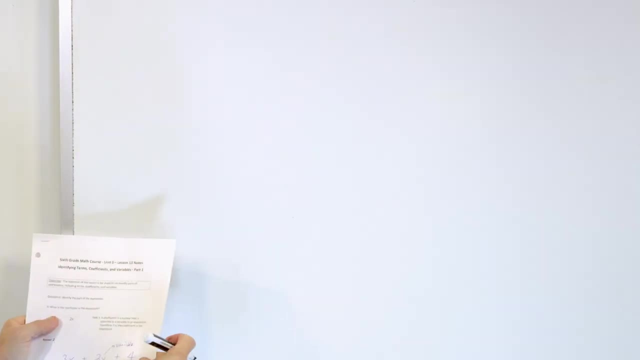 I'm going to ask you a question. So I want you to tell me- here is what I'm writing down: 2x. I want you to tell me what is the coefficient. What is the coefficient in that expression? What is the coefficient So underneath? we're going to 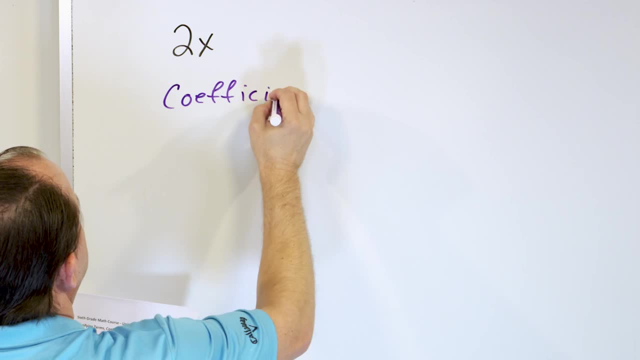 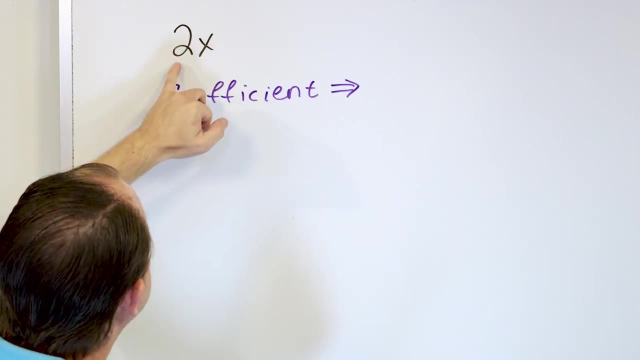 write coefficient. What is the coefficient Equal? Well, there's only one term here And we have one variable And the only number that's in front of the only thing that we have here, the number in front of variable, is a 2.. So the coefficient here is the number 2.. See how easy that was. The 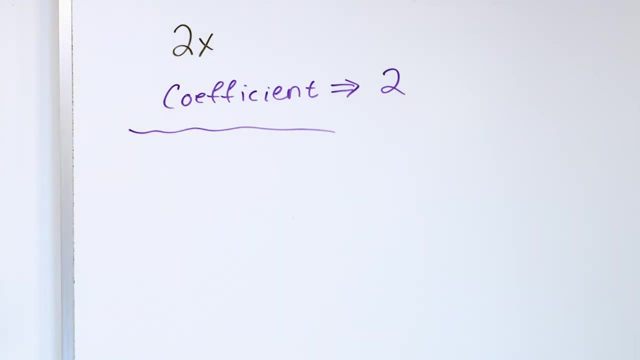 coefficient is the number in front of the variable, And so that's a 2.. All right, let's move along to problem number 2.. I'm going to write down 7x, I'm going to write down 7y, And I want you to tell me the following: I want you to tell me what is. 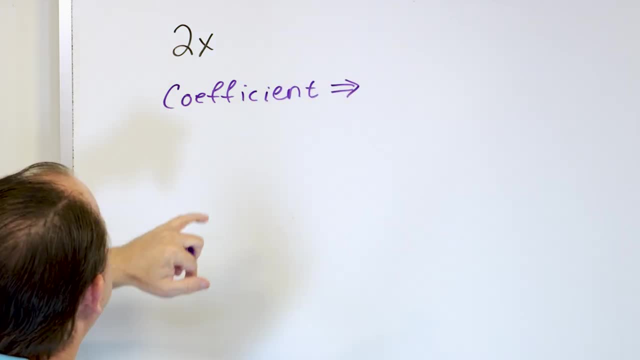 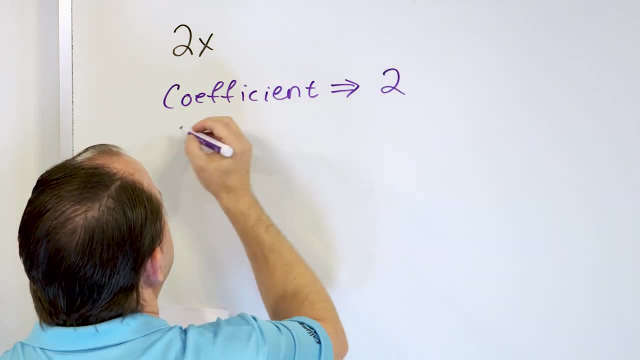 What is the coefficient equal? Well, there's only one term here and you have one variable and the only number that's in front of the only thing that we have here, the number in front of variable is a 2.. So the coefficient here is the number 2.. See how easy that was The coefficient. 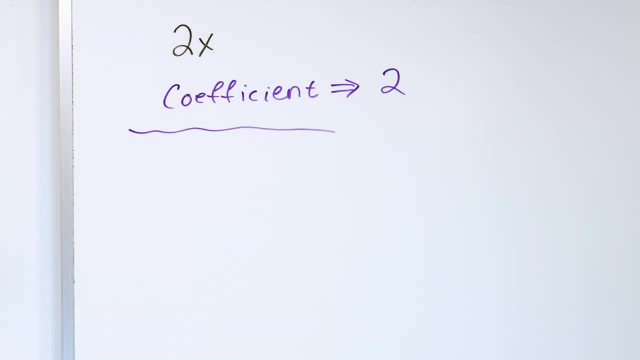 is the number in front of the variable, and so that's a 2.. All right, To move along to problem number 2, I'm going to write down 7y And I want you to tell me the following: I want you to tell me what is the variable. 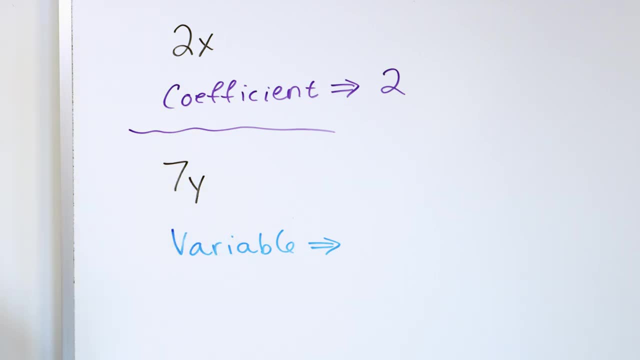 What is the variable in this expression? This is a very simple expression with one little term. What's the variable? Well, y is the letter, The variable is y, So that's it. Next problem: What about if I just give you a really, really simple term? It's just a single. 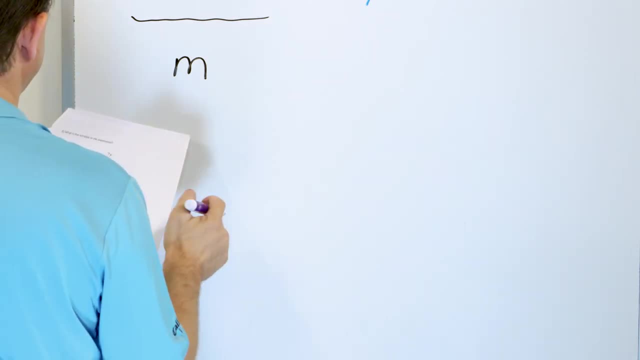 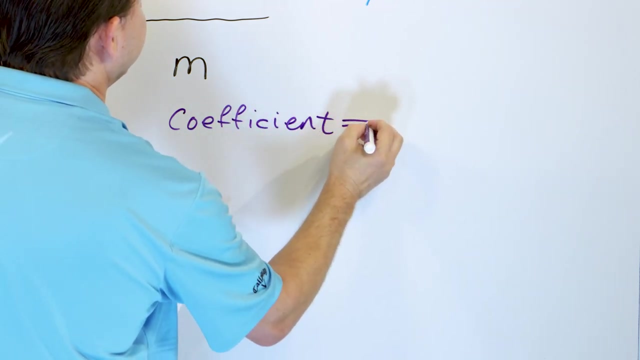 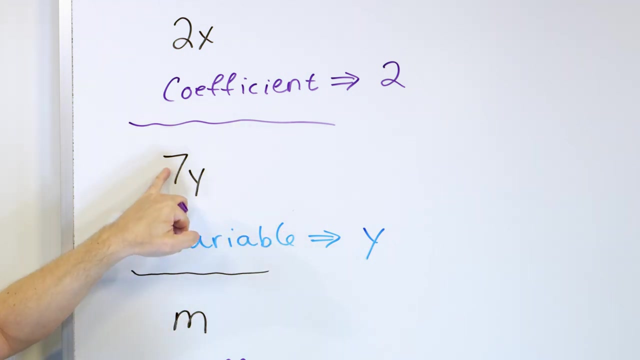 letter M And I want you to answer me the following question: What is the coefficient? What is the coefficient there? You might say: I don't see anything, There's nothing there. Remember, coefficient is the number in front, So 7. here is the coefficient in front of the Y. 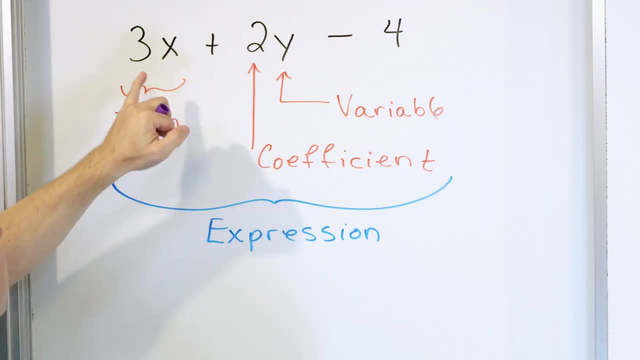 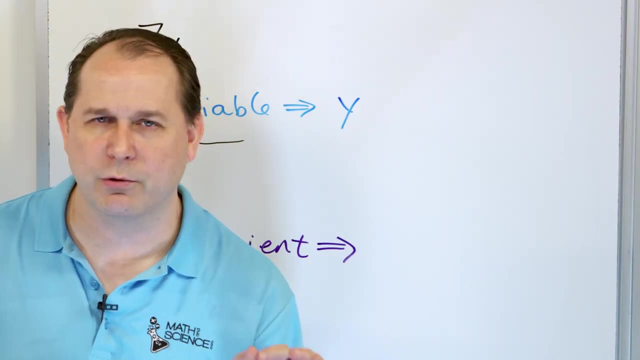 2. here is the coefficient here. 2. here is the coefficient in front of that Y. 3 is the coefficient in front of this. But in front of this M I don't see anything. So a lot of people want to write 0 down. No, it's not 0. There is a number in front of here. It's invisible, It's the number. 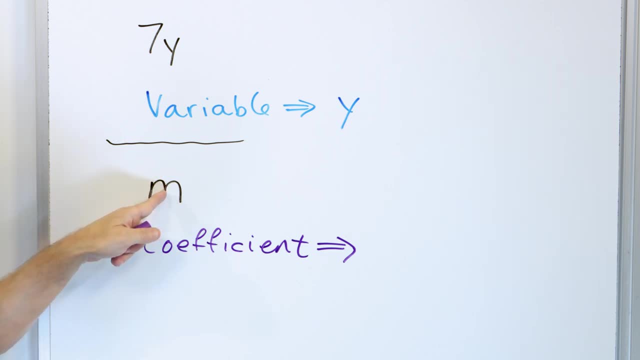 1. Because if there's an invisible 1 here, 1 times M is just M. That's what I have here. So the coefficient has to be 1.. If you think the coefficient's 0,, then if there would be an 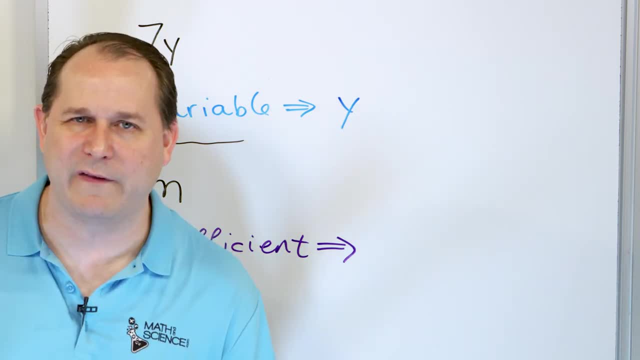 invisible 0 here, then 0 times M is 0, and there's nothing at all there. So the coefficient can't be 0.. If you just have a variable with nothing written in front of it, the coefficient is always 1, because it's M times the invisible 1. that's there. The coefficient is 0.. 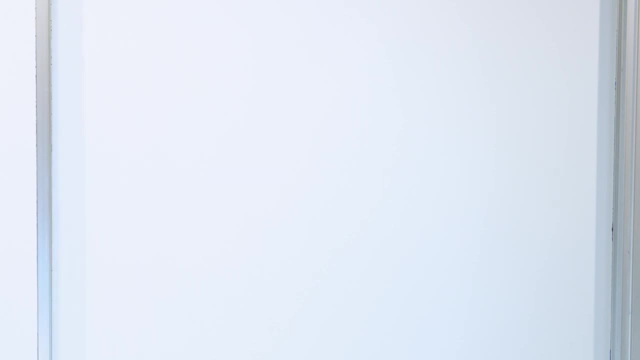 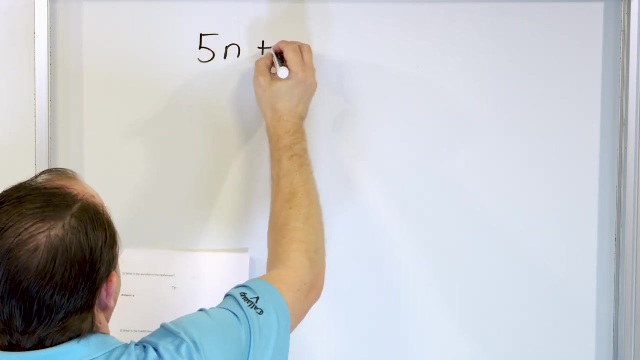 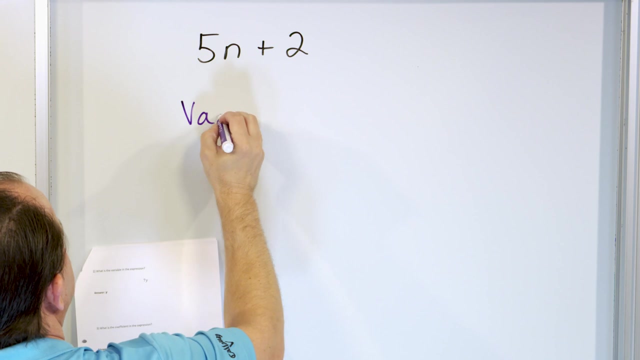 All right, Let's move right along. Let's look at something a little more complex. What about 5n plus 2?? So that's the expression, And underneath we want to answer the following question: What is the variable? What is the variable here? Well, there's no variable here. The only letter I see is: 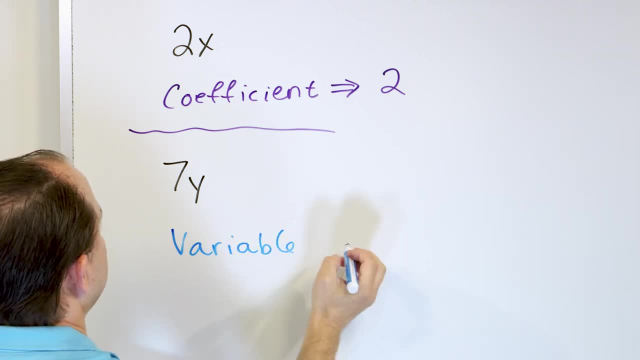 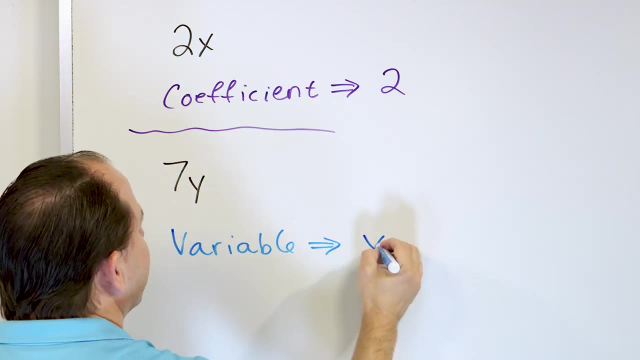 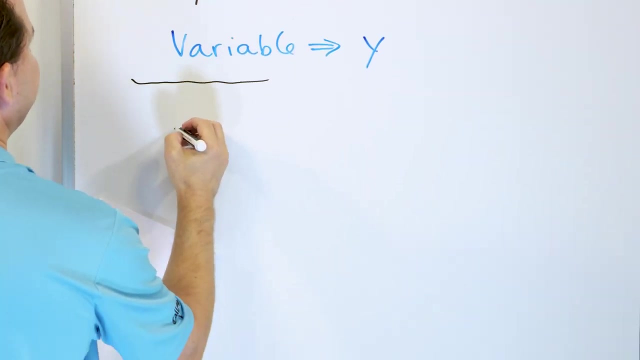 the variable. What is the variable in this expression? This is a very simple expression with one little term. What's the variable? Well, y is the letter, The variable is y, So that's it All right. next problem: What about if I just give you a really, really simple term? It's just a. 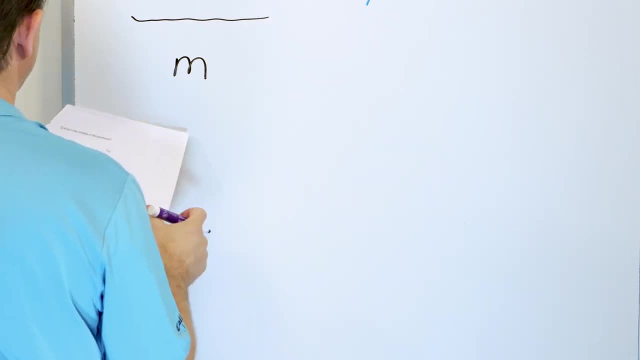 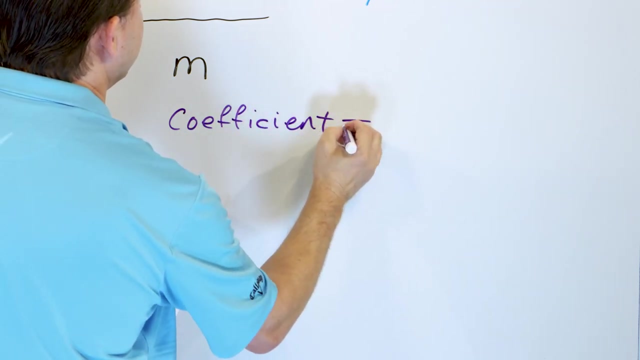 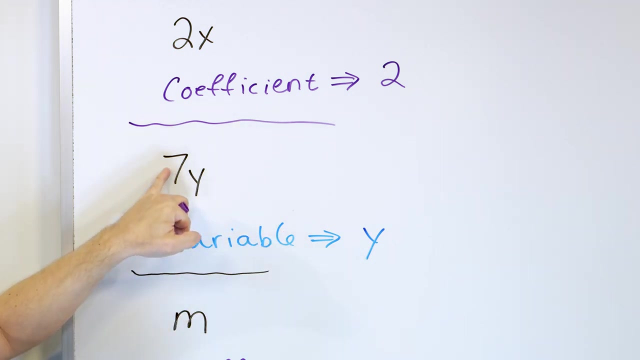 single letter m And I want you to answer me the following question: What is the coefficient? What is the coefficient there? You might say: I don't see anything. There's nothing there. Remember, coefficient is the number in front, So 7. here is the coefficient. 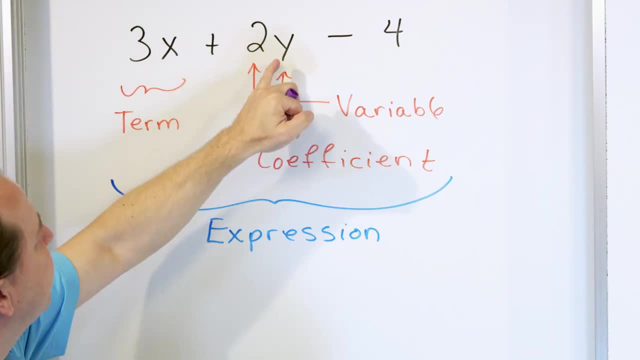 in front of the y 2. here is the coefficient here. 2. here is the coefficient in front of that y. 3 is the coefficient in front of this. But in front of this m I don't see anything. So a lot of people. 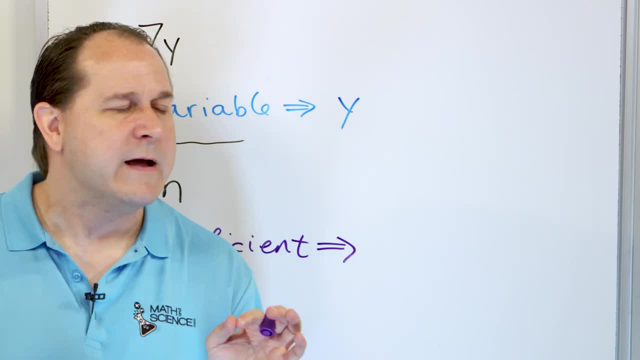 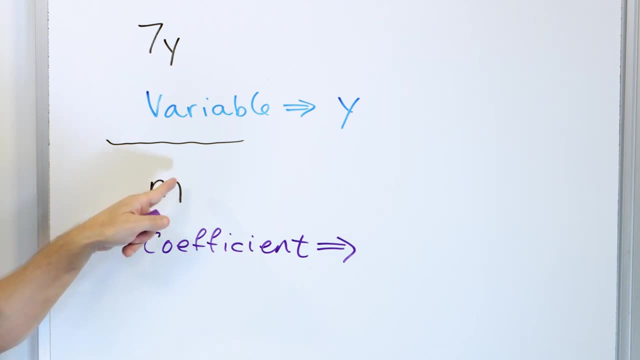 want to write 0 down. No, it's not 0.. There is a number in front of here. It's invisible, It's the 1.. Because if there's an invisible 1 here, 1 times m is just m. That's what I have here. So the 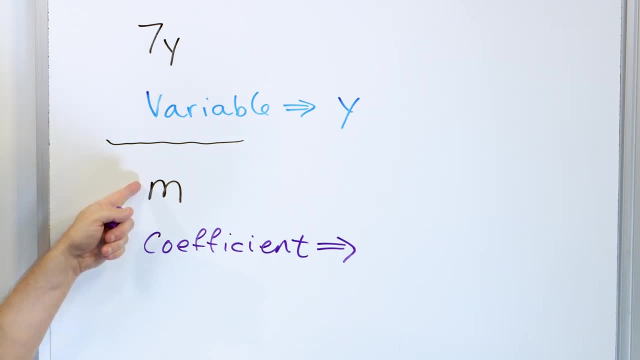 coefficient has to be 1.. If you think the coefficient is 0,, then if there would be an invisible 0 here, then 0 times m is 0. And there's nothing at all there. So the coefficient can't be 0. If you just 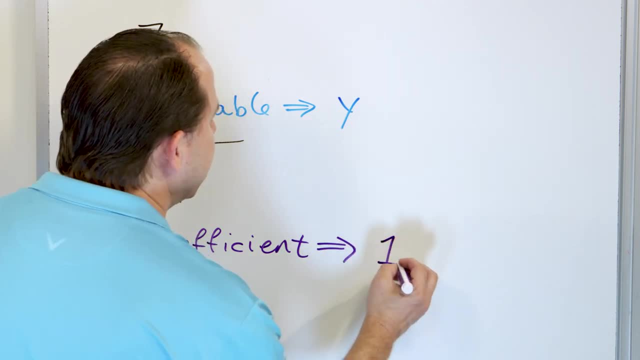 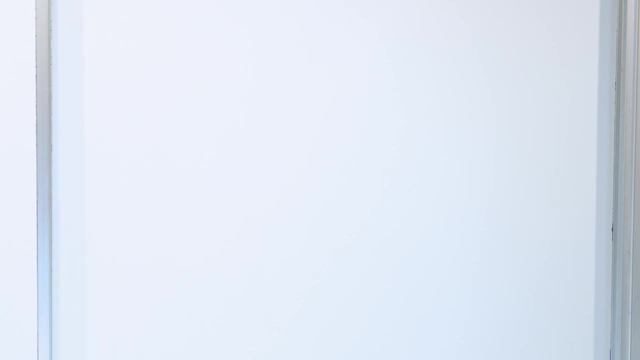 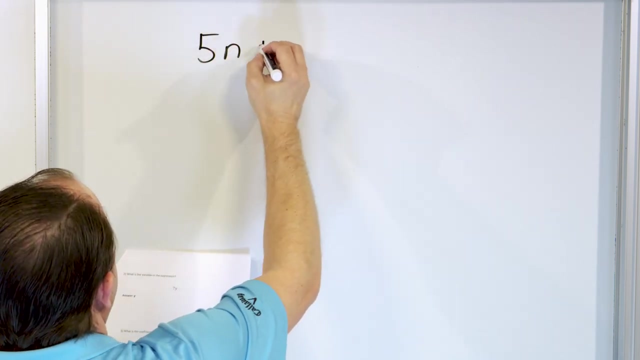 have a variable with nothing written in front of it, the coefficient is always 1.. Because it's m times the invisible 1. that's there. The coefficient of m there is 1.. All right, Let's move right along. Let's look at something a little more complex. What about 5n plus 2?? So that's the expression. 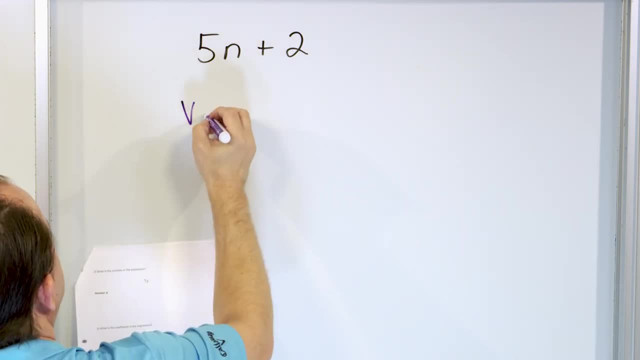 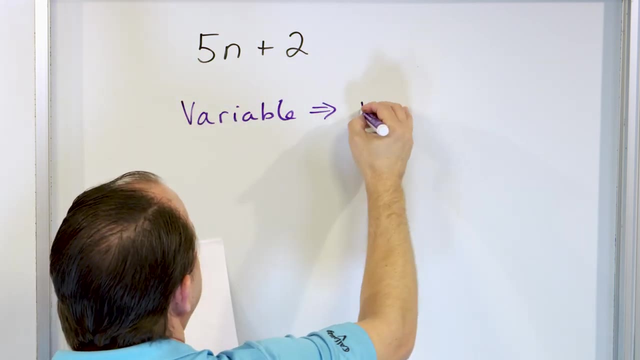 And underneath. we want to answer the following question: What is the variable? What is the variable here? Well, there's no variable here. The only letter I see is n, So the variable is n, Right, And this entire expression is 5n plus 2.. The variable is equal. 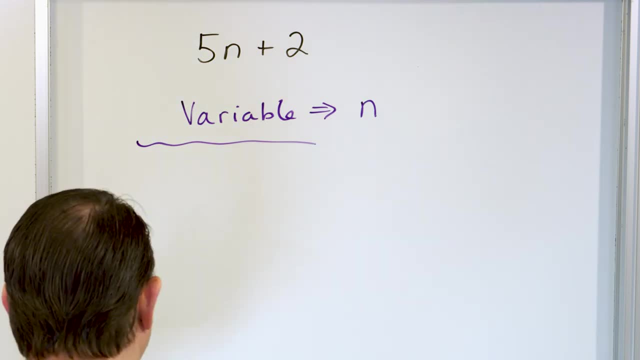 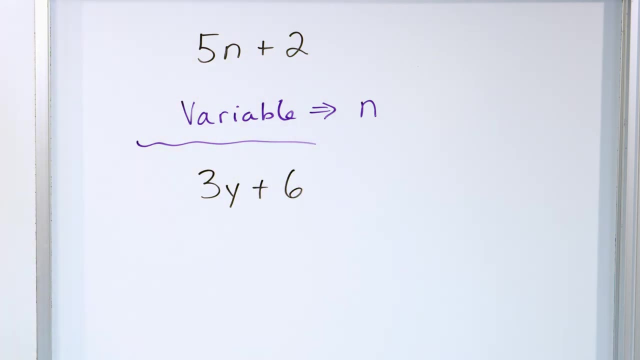 to n. All right, What else do we have? These are pretty fast, little problems. What about 3y plus 6?? And I'm going to ask you the question: what is the constant? You might say: well, he never talked about a constant. Let's go back to our original. 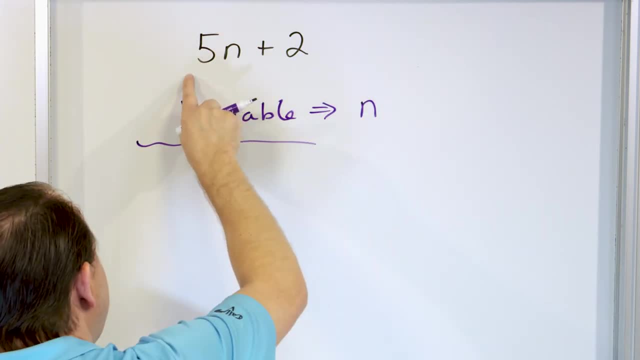 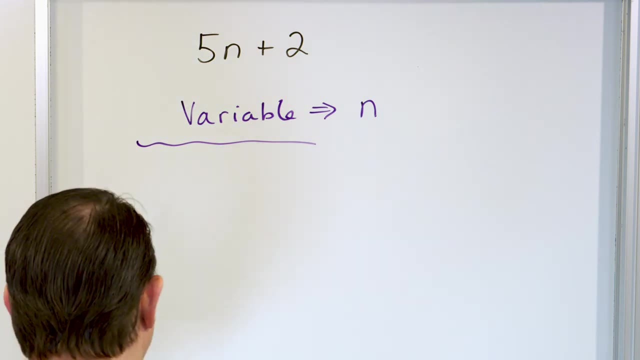 n. So the variable is n, right, And this entire expression is 5n plus 2.. The variable is equal. It's equal to n, All right, What else do we have? These are pretty fast, little problems. What about? 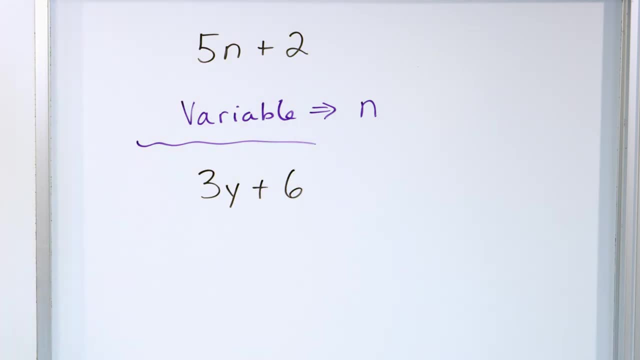 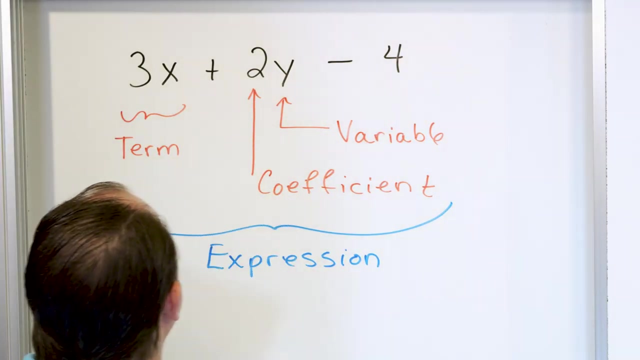 3y plus 6?. And I'm going to ask you the question: what is the constant? You might say: well, he never talked about a constant. Let's go back to our original drawing. Maybe I should add that In this expression, here was a term, Here was a term, Here is a term, This: 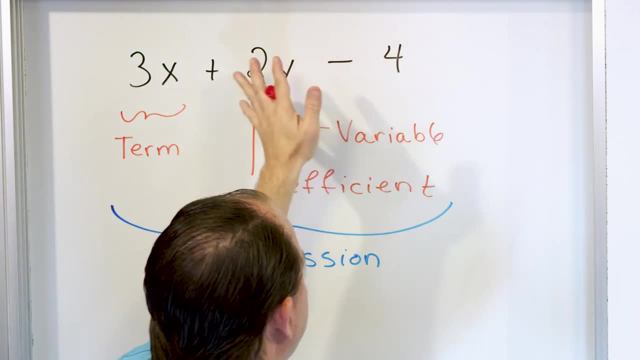 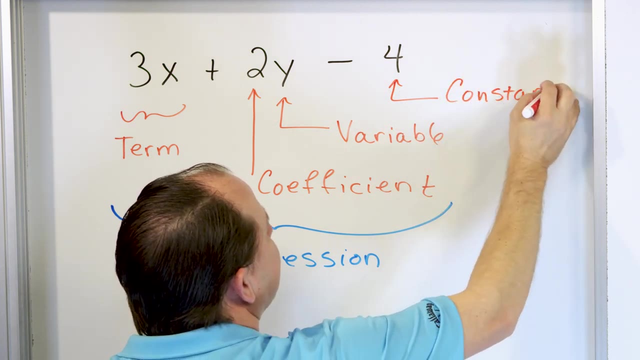 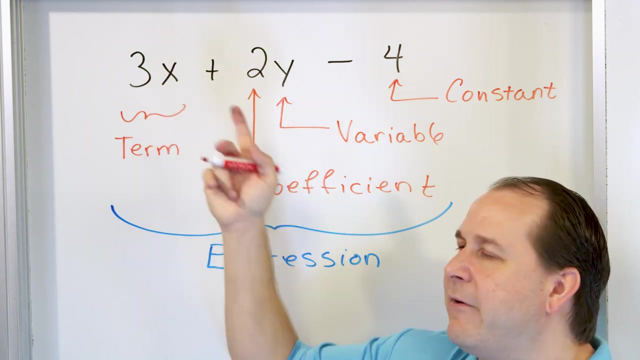 is a variable. This is a variable When we have just a number somewhere, by itself, no variables, then we can also say that this is a constant. The number constant is exactly the same meaning as just a number. A number never changes, right, All of these terms with variables. 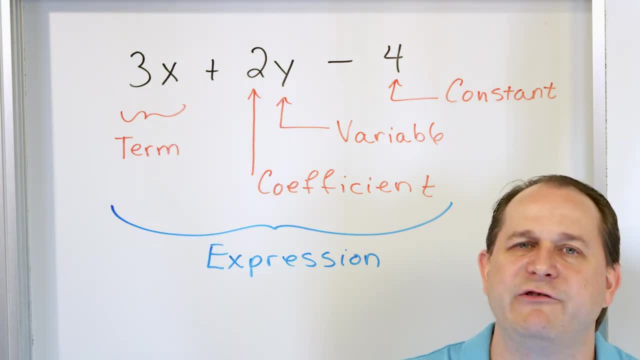 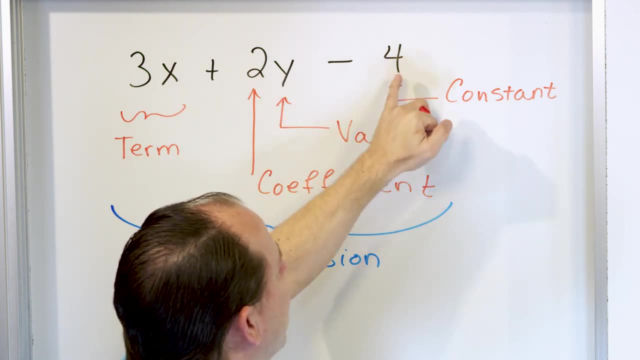 they change because when I put different numbers in for the variables then it changes what the term is when you multiply it. But no matter what happens over here, this minus 4 is going to stay the same. I call it a constant because it never changes. So when I'm over here asking you, take a look. 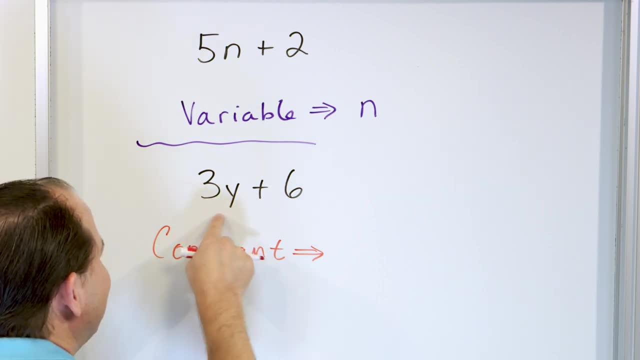 at this expression: Tell me what the constant is. It can't be this. This is changing depending on what y is The constant. is the number 6 off by itself. All right, Sorry about that. I probably should have mentioned constant there at the beginning. All right, What about the expression? 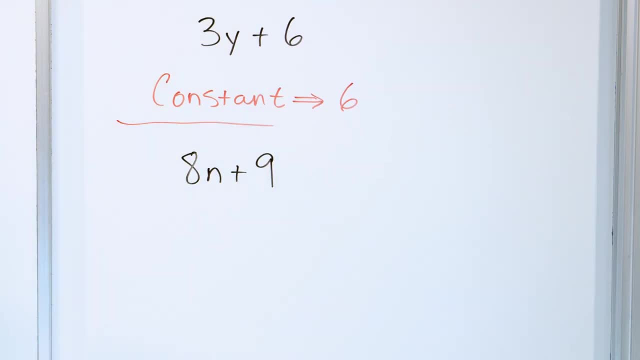 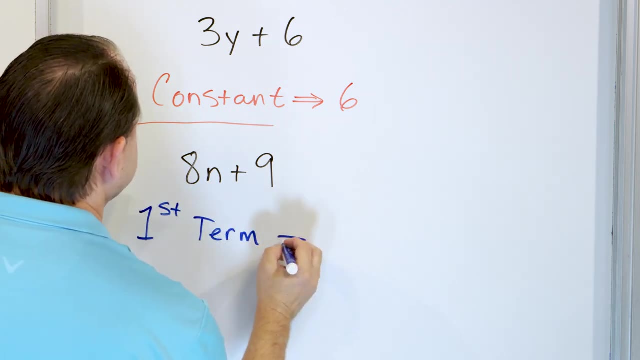 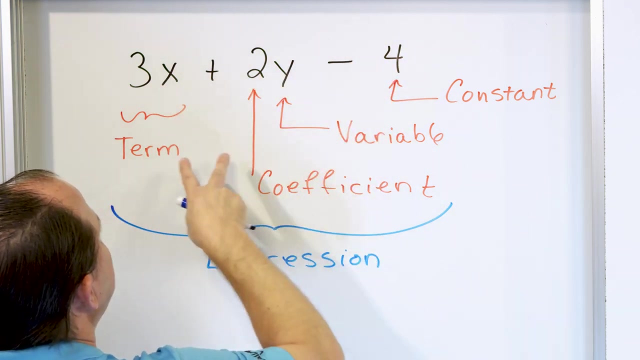 8n plus 9? And I want you to answer the following question: What is the first term in the expression? What is the first term in the expression? Remember what is a term anyway, The terms are the things that are separated by the pluses and the minuses. This is the first term. 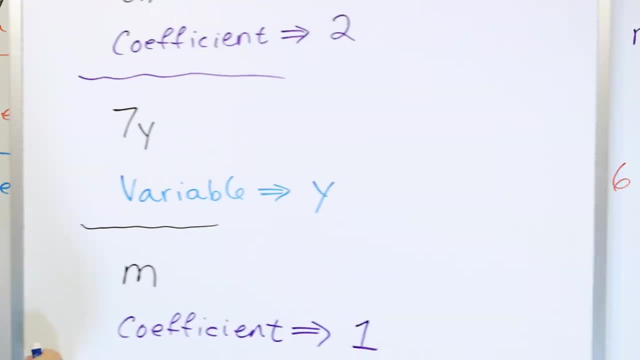 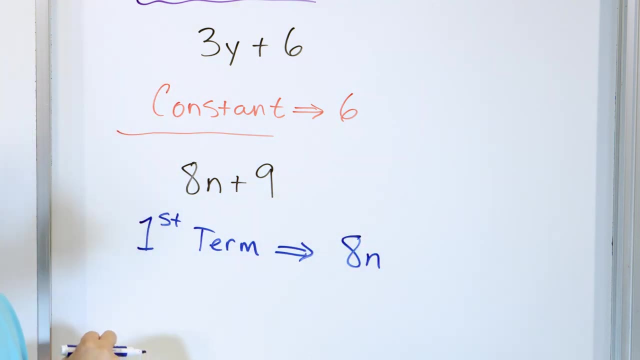 the second term, the third term. So the first term is to be whatever comes first before the plus sign. This is the first term, This is the second term. So 8n, 8 times n. Remember, when you don't have all of these, there's no multiplication symbol. It means 5 times n. 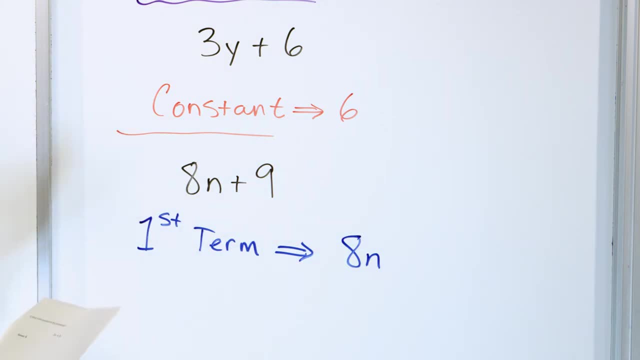 3 times y, 8 times n. So 8n, 8 times n is what we call the first term. The second term would be the 9.. And that one right there. All right, Let's take a look at. 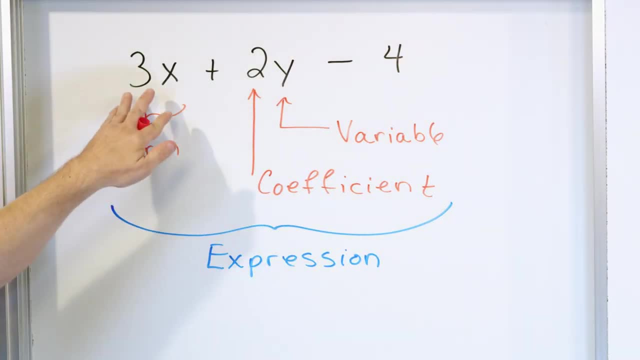 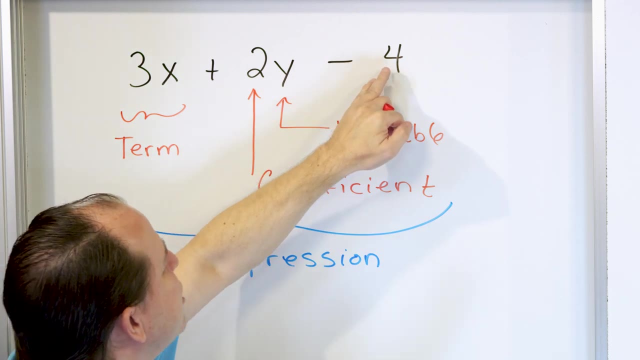 drawing. Maybe I should add that In this expression- here was a term, Here was a term, Here is a term, Right, This is a variable. This is a variable. When we have just a number somewhere, by itself no variables, then we can also say that this is a. 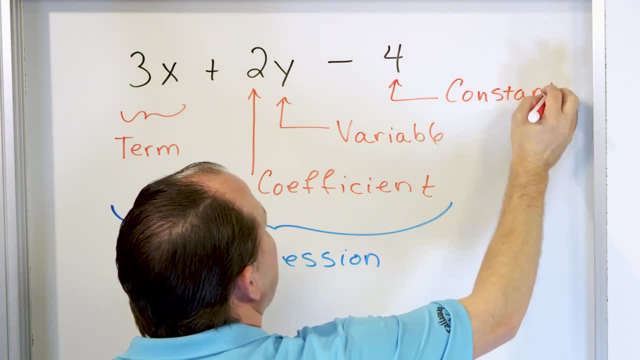 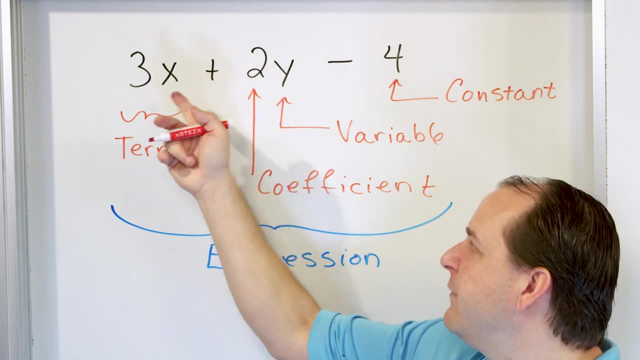 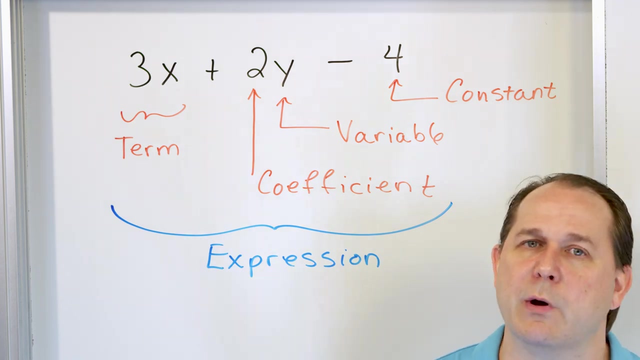 constant, The number. constant is exactly the same meaning as just a number. A number never changes, right All of these terms with variables they change because when I put different numbers in for the variables then it changes them: what you, what the term is when you multiply it. But no matter what happens over here, 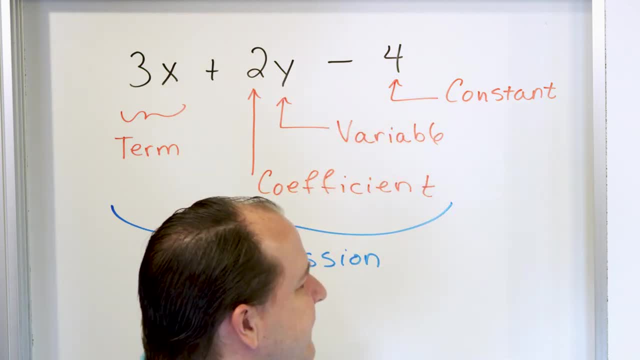 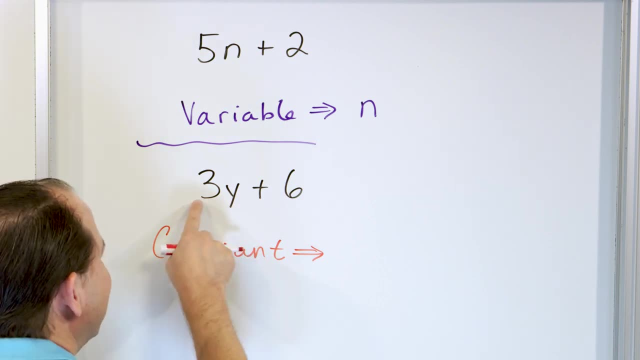 this: this minus 4 is gonna stay the same. we call it a constant because it never changes. So when I'm over here asking you, take a look at this expression, tell me what the constant is. It can't be this: This is changing depending on what y is. 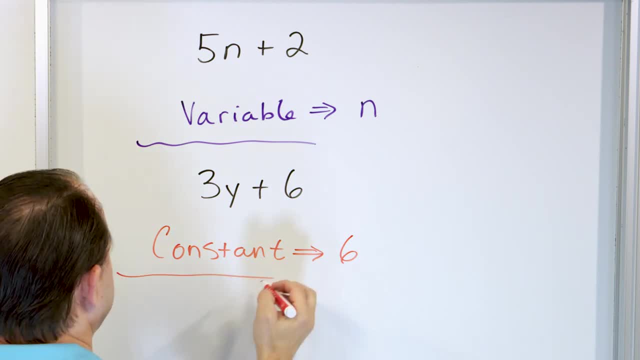 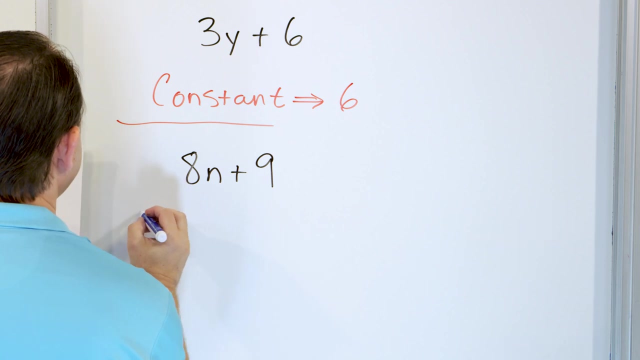 The constant is the number 6 off by itself. All right, sorry about that. Probably should have mentioned constant there at the beginning. All right, what about the expression 8n plus 9?? And I want you to answer the following question: What is the first term in the expression? What is the first term in the? 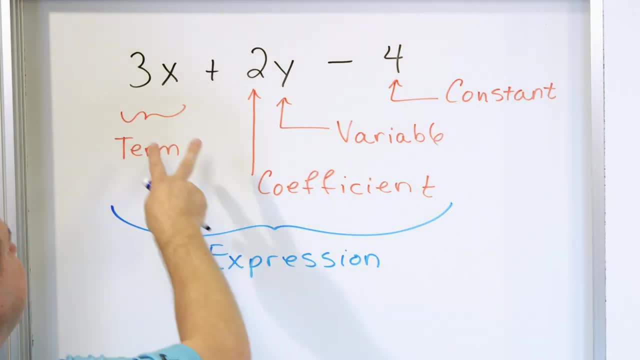 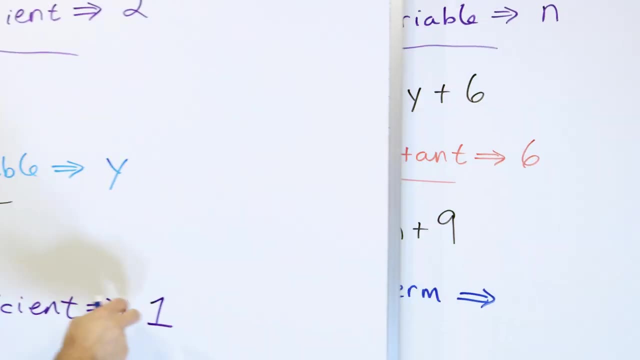 expression. Remember what is a term? anyway, The terms are the things that are separated by the pluses or the minuses. This is the first term, the second term, the third term. So the first term is to be whatever comes first before the. 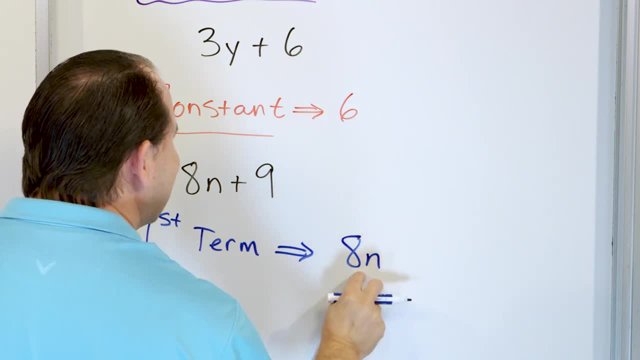 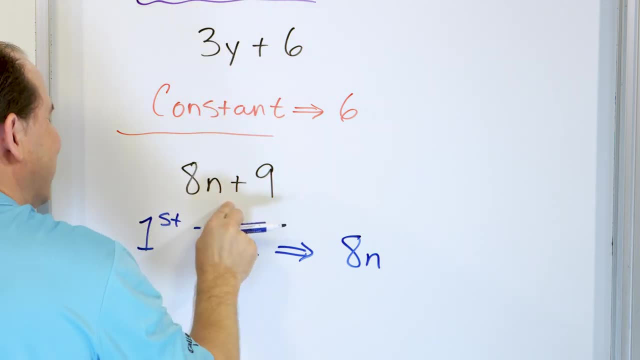 plus sign. This is the first term. This is the second term. So 8n, 8 times n. Remember, when you don't have all of these, there's no multiplication symbol. It means 5 times n, 3 times y, 8 times n. So 8n, 8 times n is what we call the 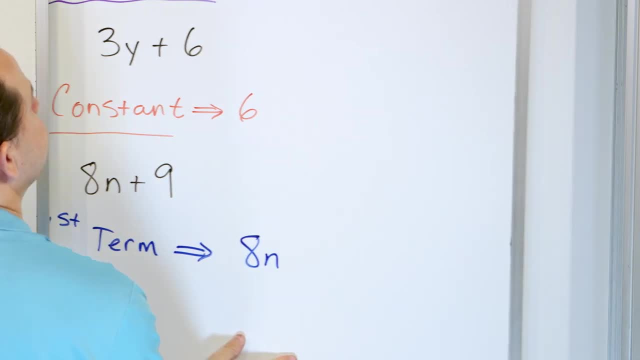 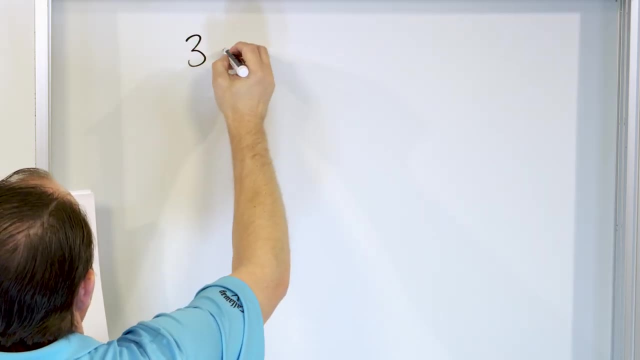 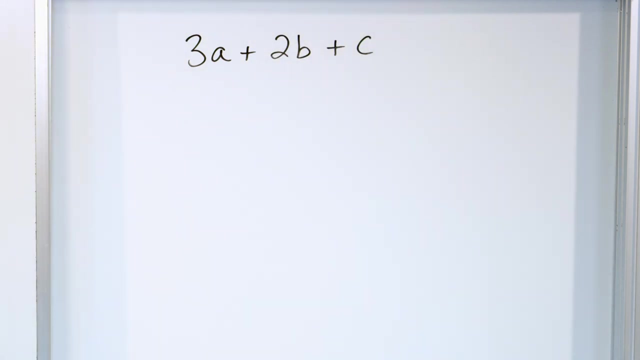 first term. The second term would be the 9.. And that one right there. All right, let's take a look at something a little more complex: 3 times a plus 2 times b plus c, And I want you to answer the following question: Name all. 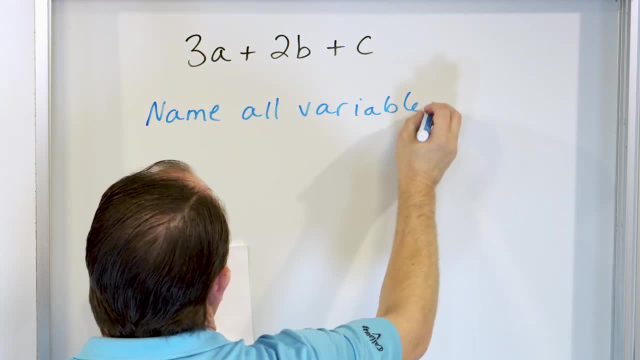 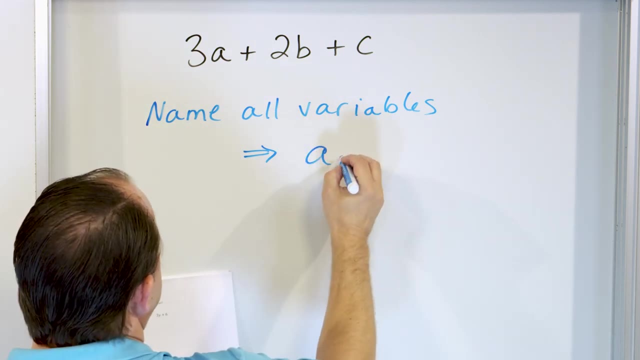 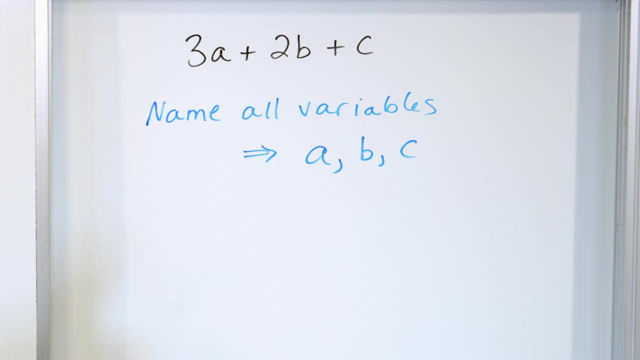 variables. All right name, all variables. Well, I see a, I see b, I see c. Basically, you're looking for all of the letters. a is a variable, b is a variable, c is a variable. Right, What would the first term be? This would be the first term. What would the? 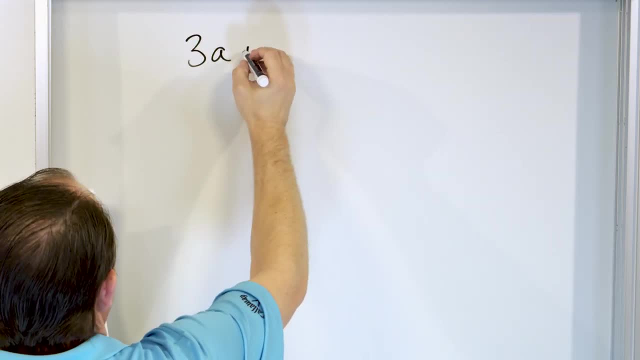 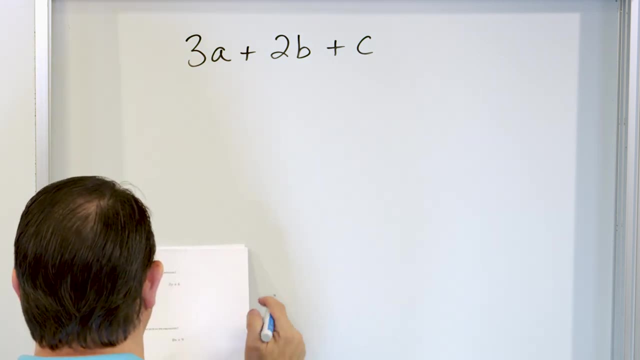 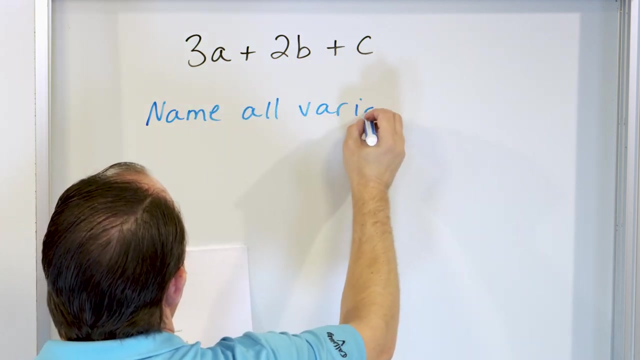 something a little more complex: 3 times a plus 2 times b plus c. And I want you to answer the following question: Name all variables? All right, Name all variables. Well, I see A, I see B, I see C. 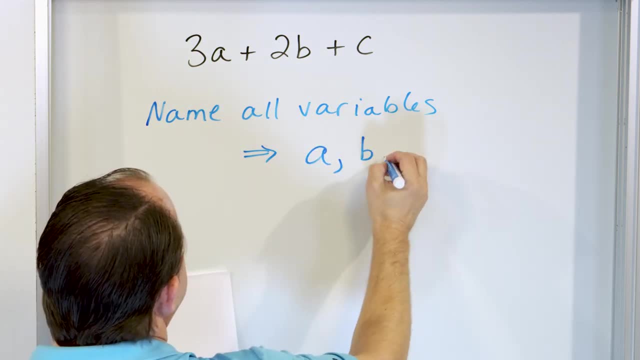 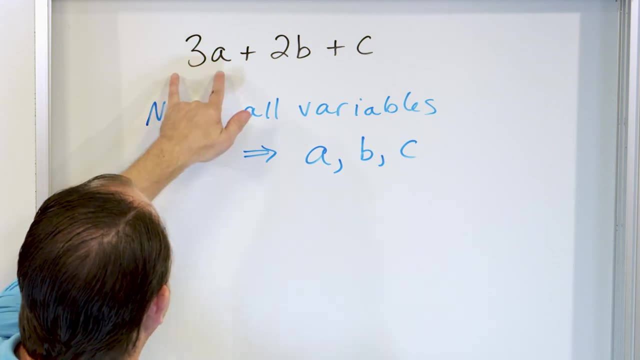 Basically, you're looking for all of the letters: A is a variable, B is a variable, C is a variable right. What would the first term be? This would be the first term. What would the third term be? It would be this one right. 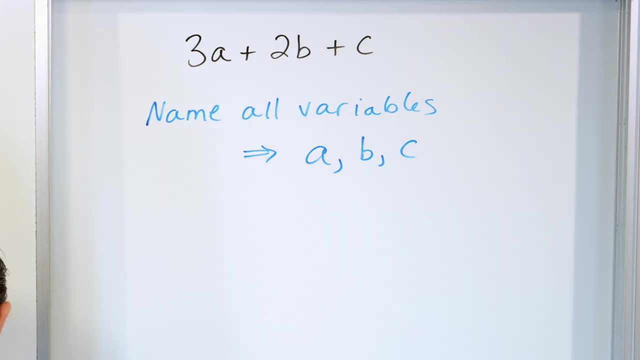 Stuff like that. We can just kind of move along and do some more problems. but I'm just trying to kind of make up a little more as we go to give you more practice. Almost done. Take a look at 16 plus 3 times X plus 4 times Z. 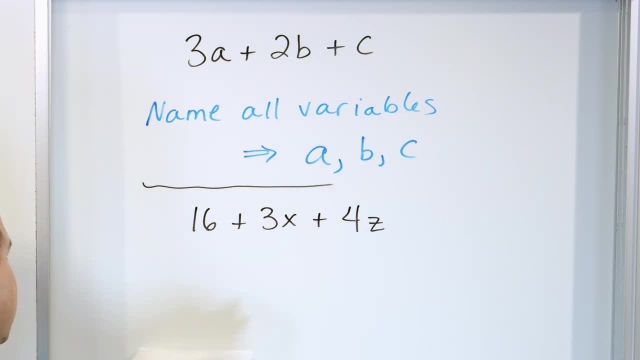 And we want to ask ourselves the question name all, I'm sorry, name the variable of the second term. So we're going to ask ourselves: what is the variable? The A-R is variable in the second term. What is it? 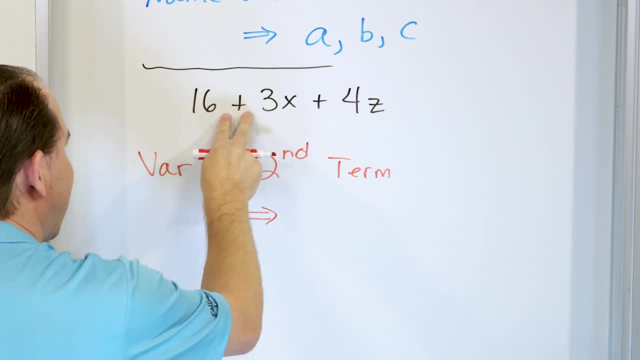 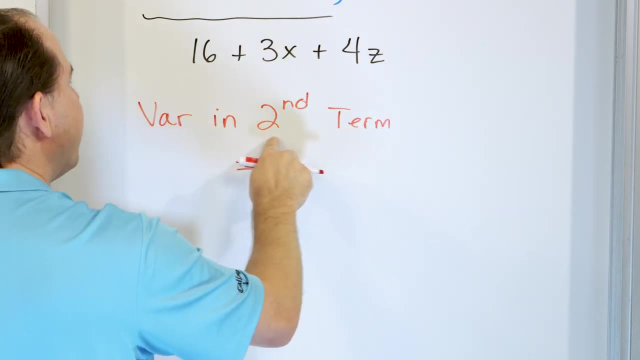 So where is the second term? This is the first term. It's linked by a plus sign with the second term, linked by a plus sign with the third term. So the second term is this one. The variable in the second term is the letter that you see. 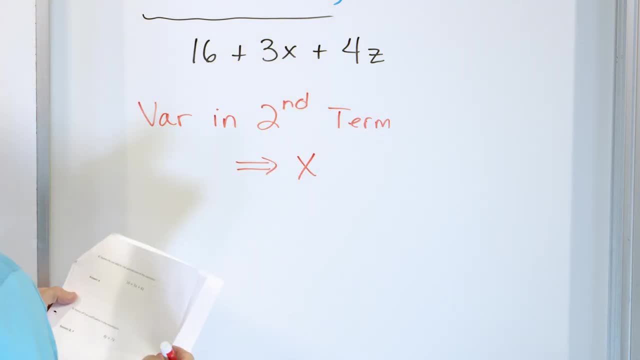 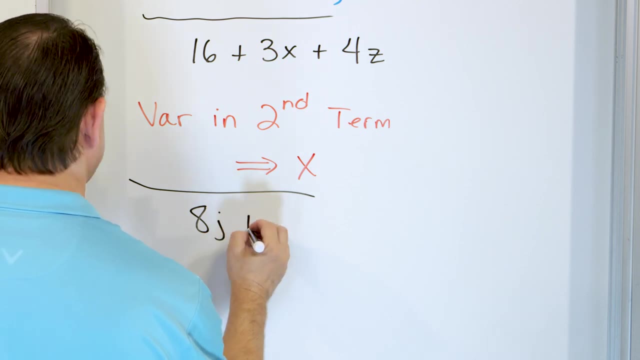 in the second term. so it's got to be X. So that's the answer there: X. All right, only two more. We're going to write down 8 times J plus 7 times K And we're going to ask ourselves the following question: 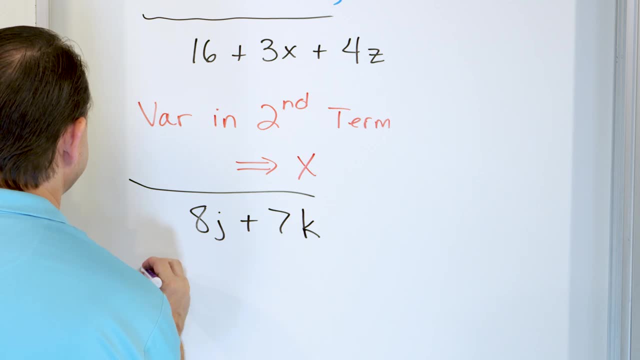 8J plus 7K. Name all coefficients. Coefficients- I'm going to abbreviate coefficients, as you see right there. So the coefficient of the first term is 8, and the coefficient of the second term here is 7.. 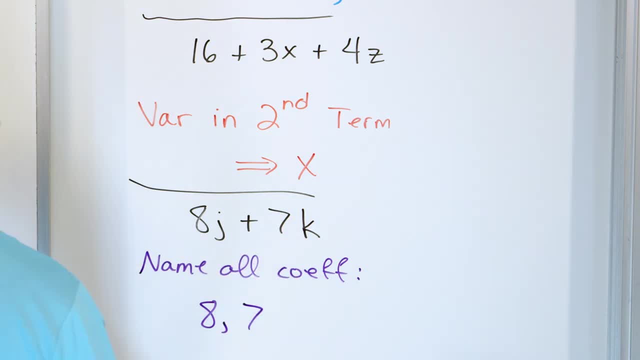 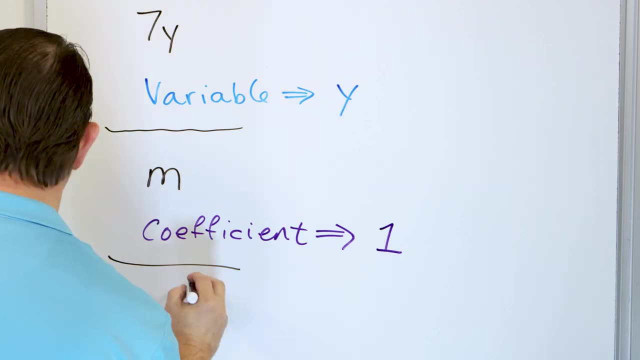 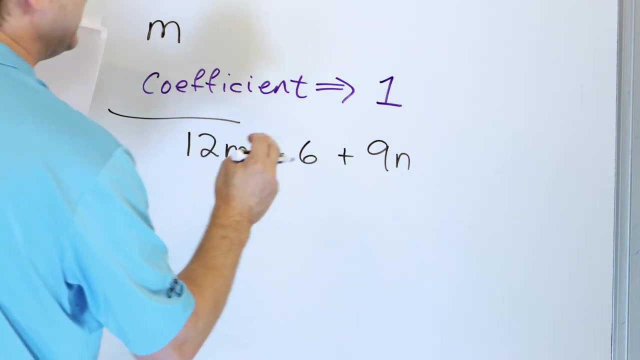 So 8 and 7 are all of the coefficients that we have right there, And I think I'm going to squeeze back over here to do my very last problem. Well, let's write down 12 times M plus 6 plus 9 times N. 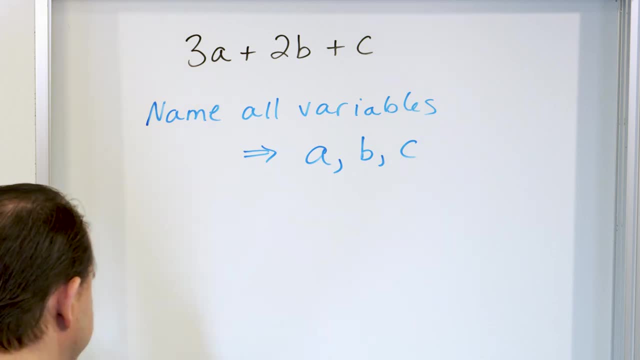 third term be. It would be this one Right Stuff like that. We can just kind of move along and and do some more problems. But I'm just trying to kind of make up a little more as we go to give you more practice. Almost done, Take a. 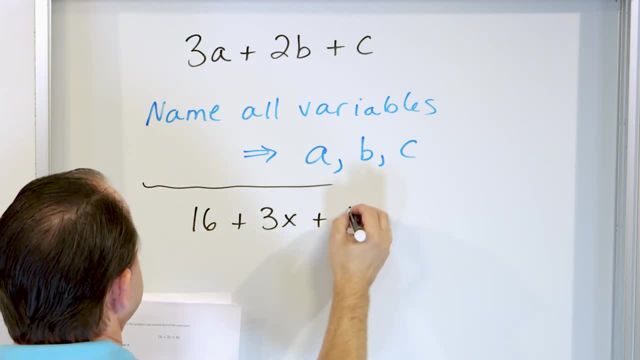 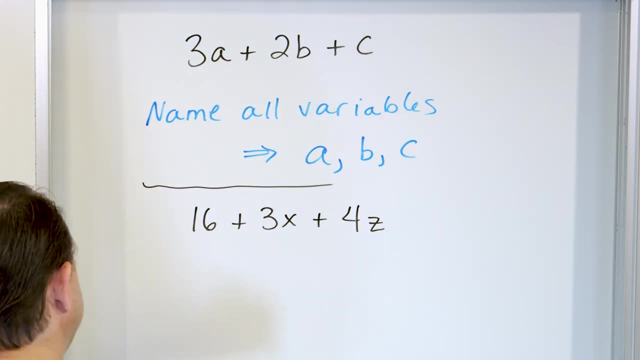 look at 16 plus 3 times x plus 4 times z, And we want to ask ourselves the question: Name all, I'm sorry name the variable of the second term. So we're going to ask ourselves: what is the variable? the a- r is variable in the second term. What is it? So? where is the? 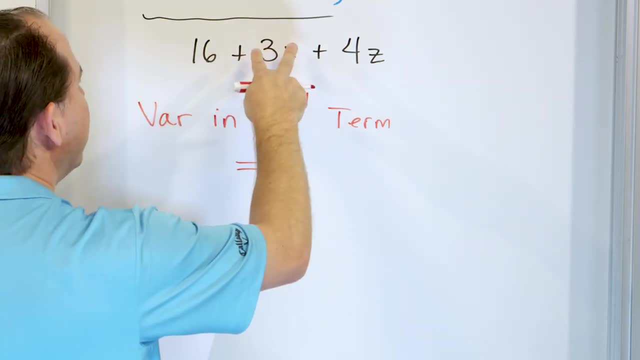 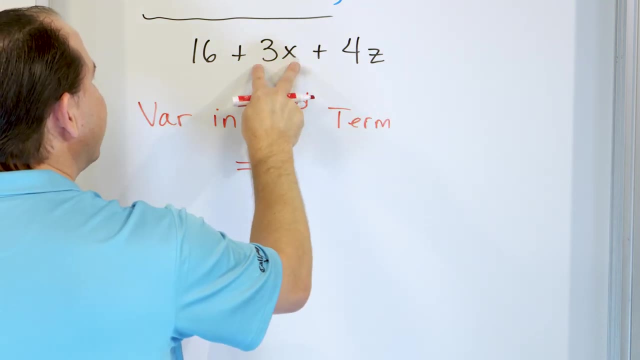 second term. This is the first term. It's linked by a plus time with plus sign with the second term, Linked by a plus sign with the third term. So the second term is this one. The variable in the second term is the letter that you see in the. 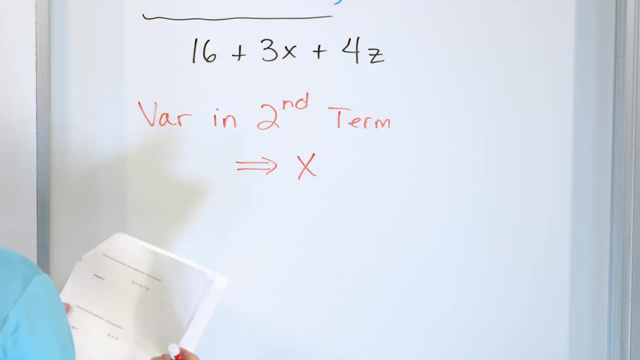 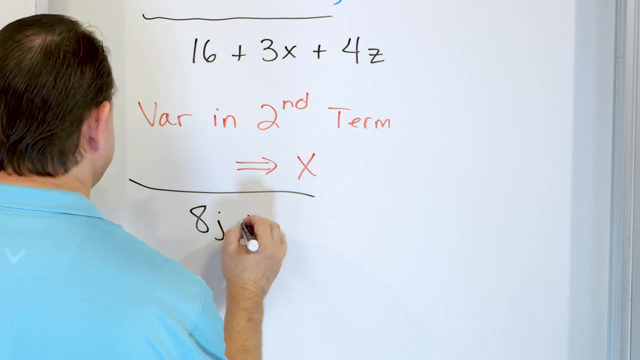 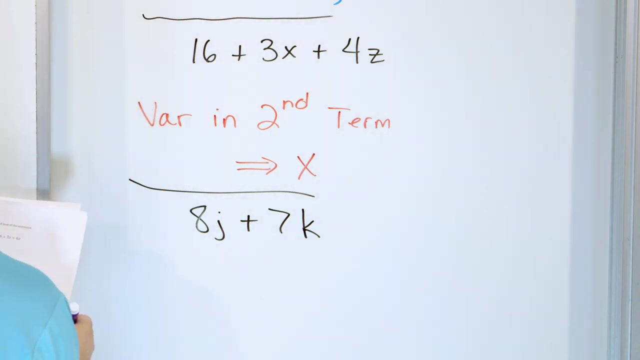 second term. So it's got to be x. So that's the answer there: x. All right, Only two more. We're going to write down 8 times j plus 7 times k And we're going to ask ourselves the following question: 8j plus 7k, Name all. 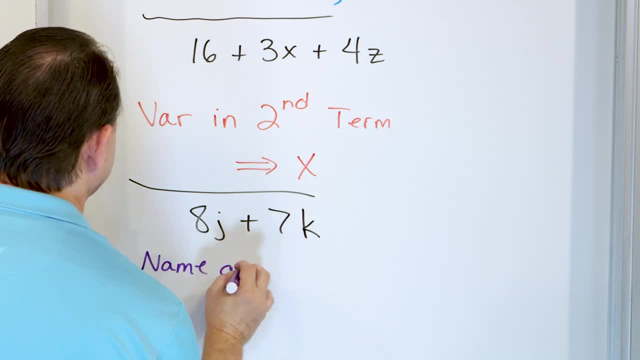 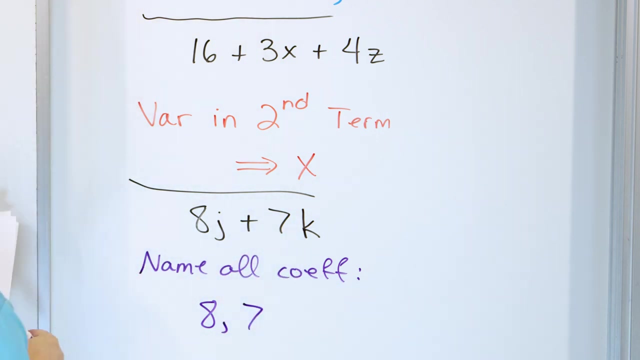 coefficients, Coefficients- I'm going to abbreviate coefficients, as you see right there. So the coefficient of the first term is 8 and the coefficient of the second term here is 7.. So 8 and 7 are all of the coefficients that we have, right there. 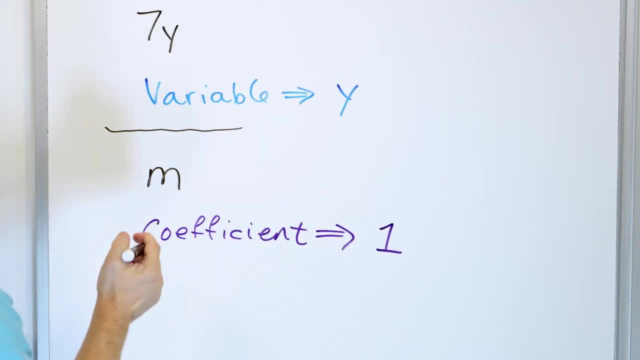 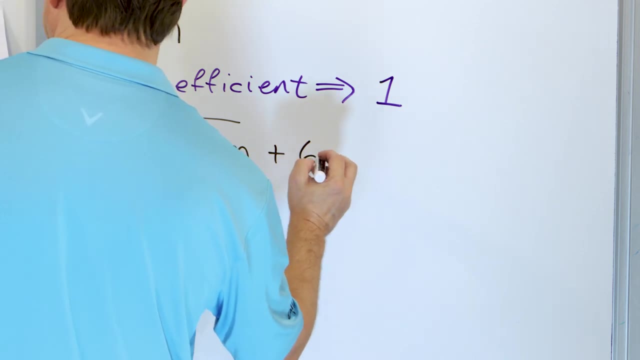 And I think I'm going to squeeze back over here to do my very last problem. Well, let's write down 12 x m plus 6 plus 9 x n, 9 x n, And we're going to ask ourselves the following question: What is the constant? 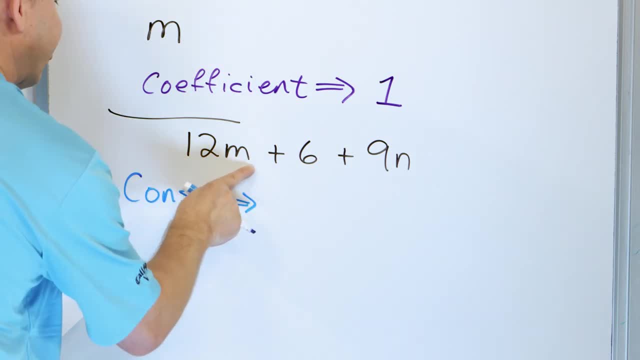 What is the constant in this expression? Well, this is the first term, And it has a variable involved. This is the second term. There is no variable. The third term has a variable involved, The only one of these terms that just has a number. the constant term is this one. So 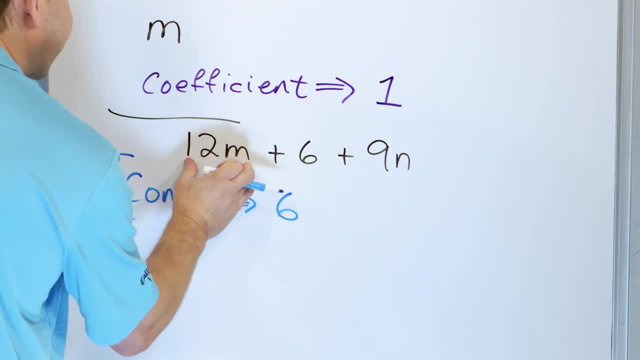 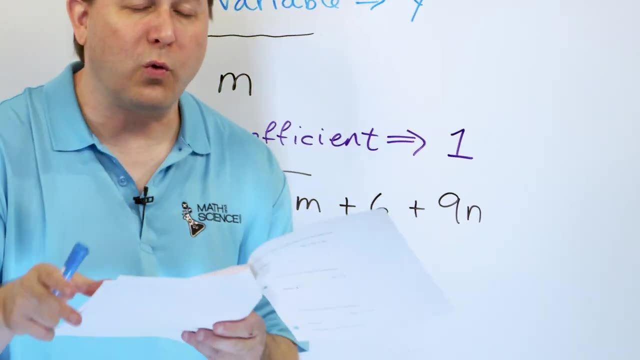 the constant is a 6. This is a variable term. This is a variable term And this one has no variable. It's a constant. It never changes. So we say the constant is 6.. So here we've learned quite a bit, Because when you first learn this stuff you have a lot of definitions hitting you.